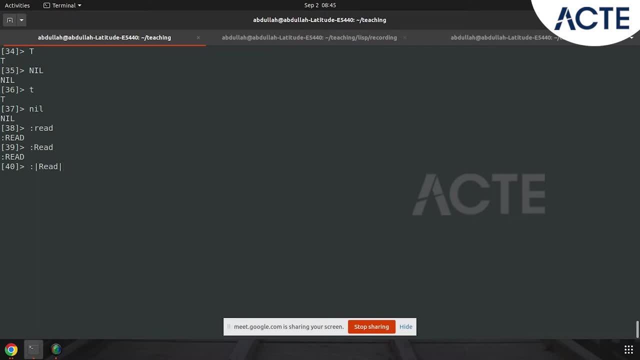 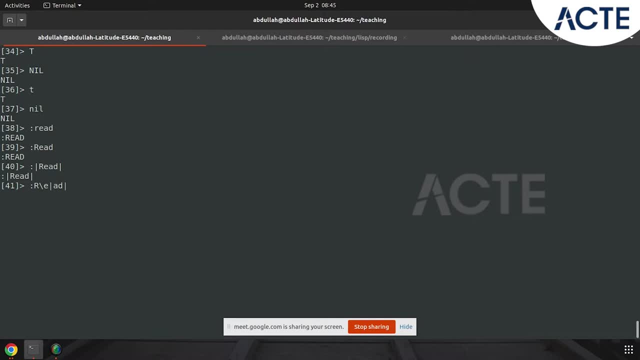 use a slash to make the to retain the missing, So the slash escapes one character, backslash escapes one character, Whereas vertical bars you can have, you know, you can place it between a string of a sequence of characters or a string, So you can escape a string, whereas 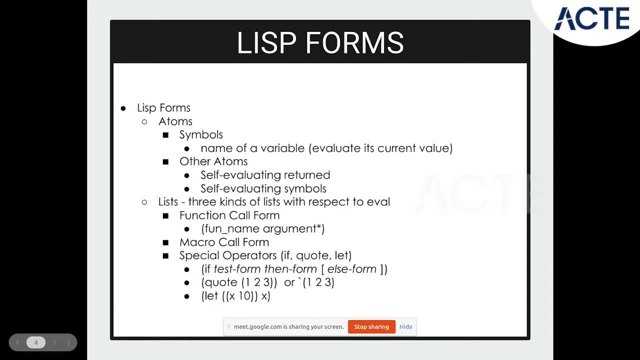 slash backslash, escapes a single character. So with that, atoms. I hope it is clear And follow me. Thank you, The list. it is either a function call, Function call form is actually a function name followed by argument star, Micro call form. we will come back to it, But is it clear? this function 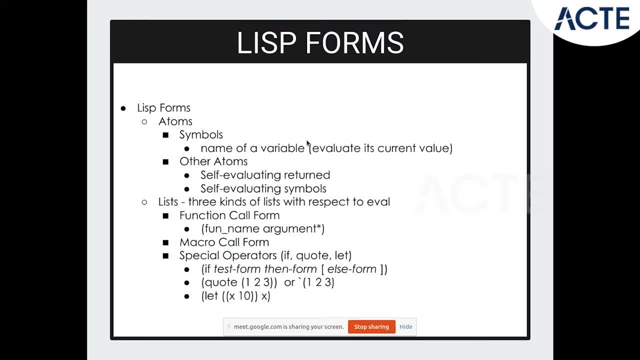 call form. So this is where we have to be clear. that we have S expression is one part of it, But you can see that a function call form has to be an S expression because it is going to be a list basically. So this is an empty list. 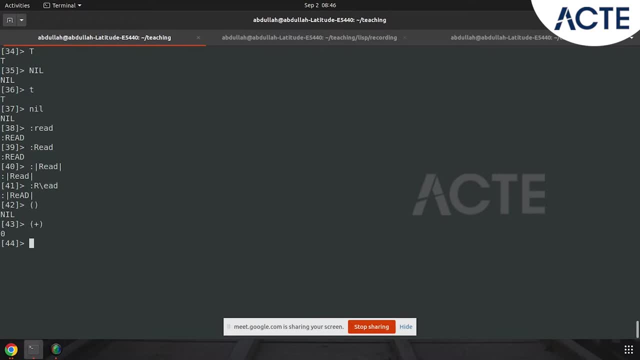 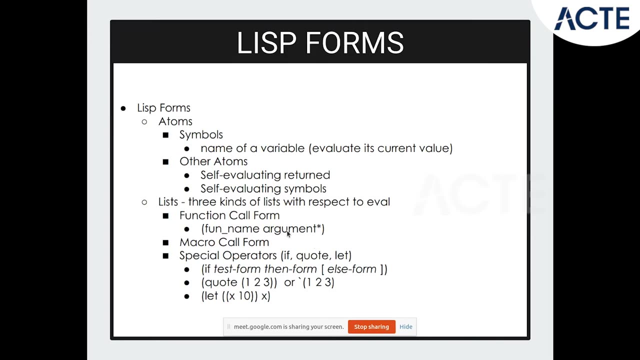 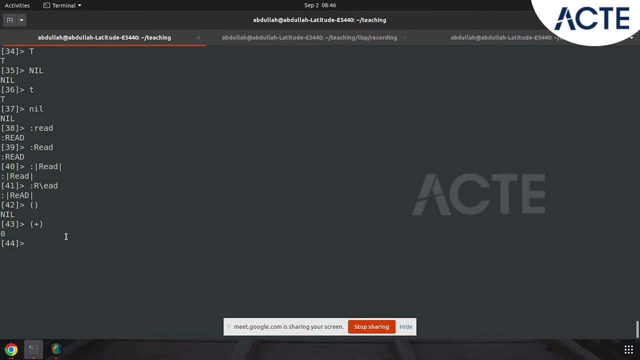 This is a function call form, All right, where plus is the and see that argument star can be one argument, It can. there can be no argument. It can be just the unary operator, like this: Okay, so this is an example of a unary operator, So plus, actually it takes. 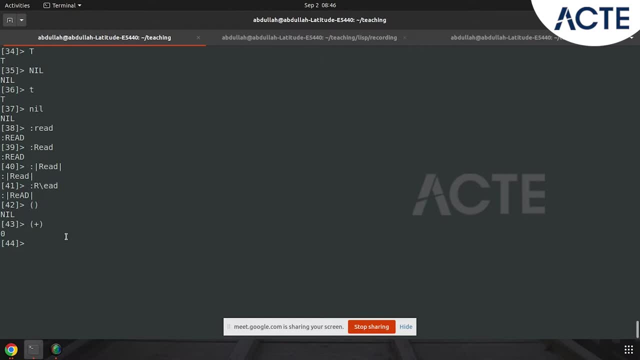 an arbitrary parameters. So plus is an example of something that takes arbitrary parameters. It can be zero, it can be one and so on. So, again, if you have the usefulness of becoming a one or you have a random operator, then it is okay. So we will come back to the table. 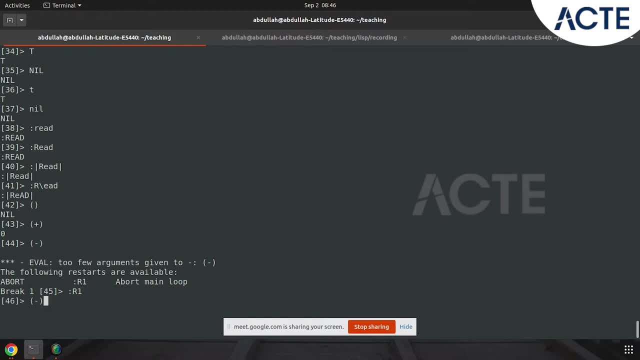 Whereas R1, my negative thing- does not have this thing. I mean it needs one argument and I want I can have one more and this is 2, so you can have like. so this is how the negative thing works. Similarly, star has this thing. it has a definition for it can. 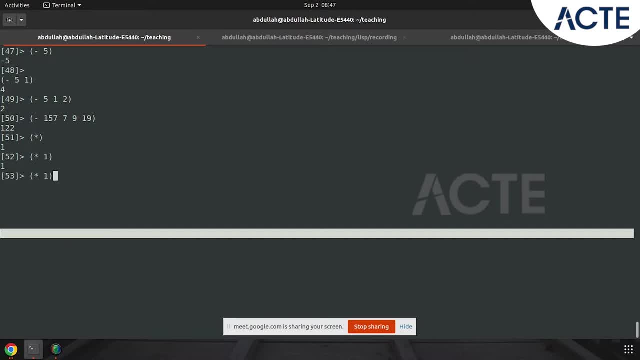 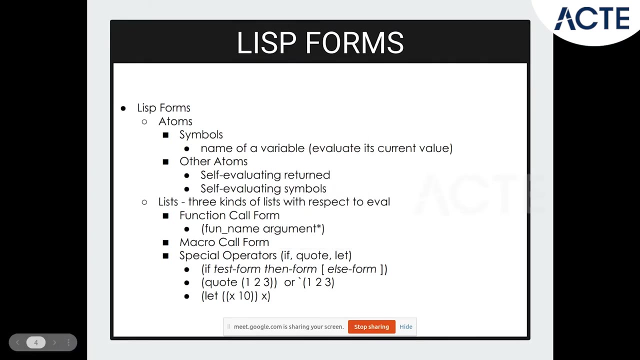 be a Euler operator, it can also be one, it can be a zero array operator, it can be considered star without parameters is actually a constant. this constant for that is just the value 1, so that is how it works. So, basically, a function called form is of this form. it is a list which has the value. 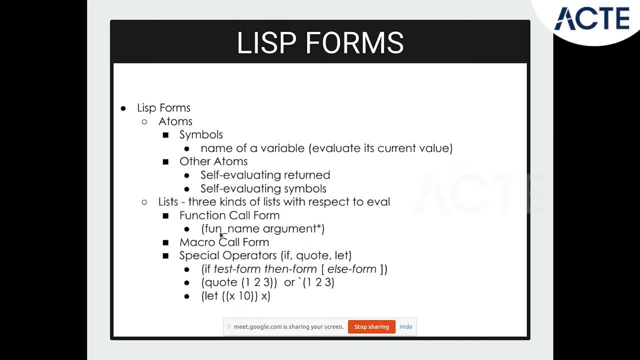 1, the first part is in the function name. this is what we were insisting that S-expressions are, but the fact is that a function called form will have it has to be an S-expression, but not every S-expression needs to be a function called form. this is the distinction that 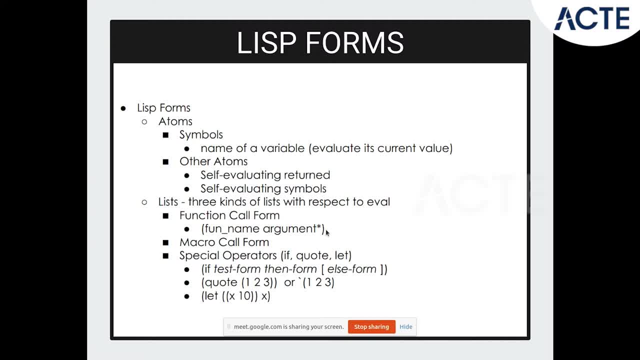 I think we have to. we have to clarify and be very clear on that, because S-expression is much more general and we can use that for defining data and for doing many things. Function- but how does it work? Function, called form, is the predominant or the most important aspect of the list, and 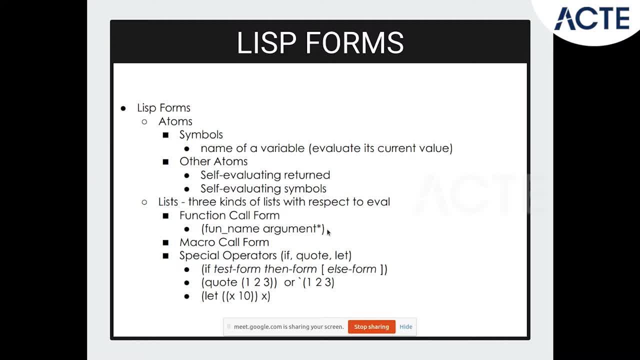 this will be used. functions are used a lot and this is what we will be discussing today in this course, in this lecture today. So majority of the thing is, if you have understand function called forms, you will be able to do a lot of things. in this you can do a lot of stuff, and in the function called form, 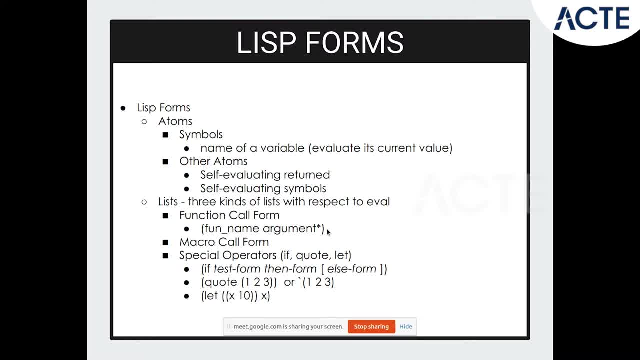 there will be parts where you will have to distinguish between places where this is a S-expression or a S-expression. so you can see that here, at this place, I need a list form and at this place I need a S-expression. it does not have to be a list form, so that 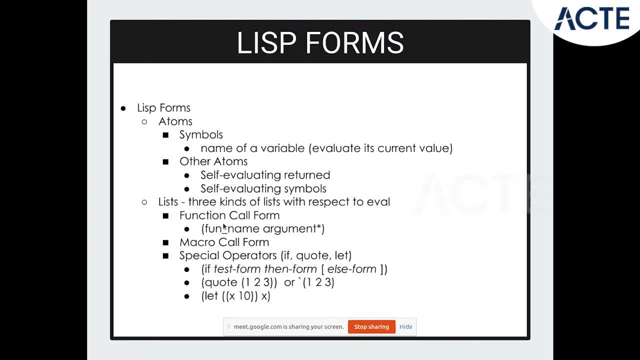 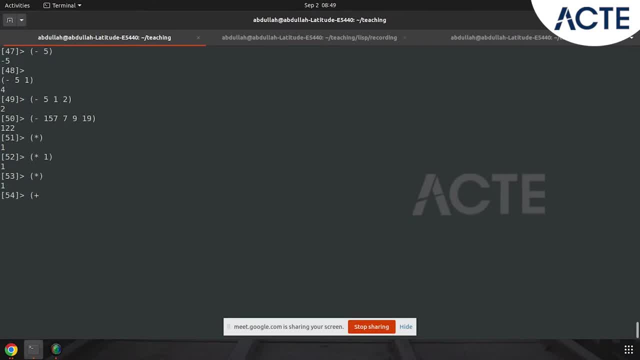 distinction is necessary to have. So for, in this example, let us just go with the function called form for plus. so for plus, this is the valid function called form. but if there is more than one argument, so let us say there is like one. 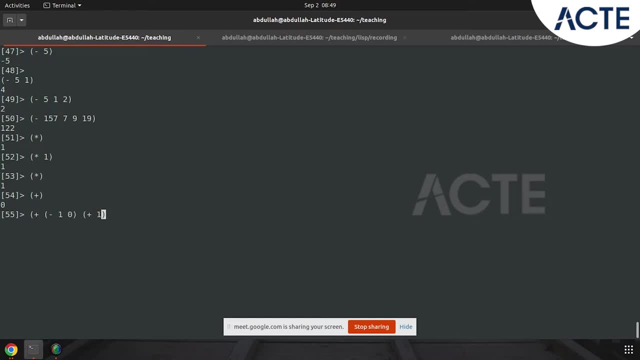 So plus, plus, plus, plus, plus. Now what happens here is the arguments for this plus. each of them should be a list form. it should be a valid list form. It can also be a special operator, but it has to be a list form. it can be like if one. 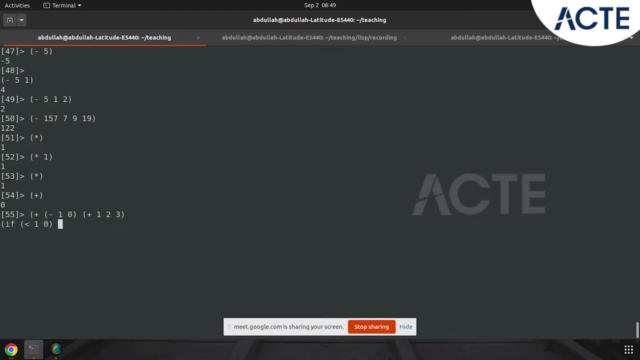 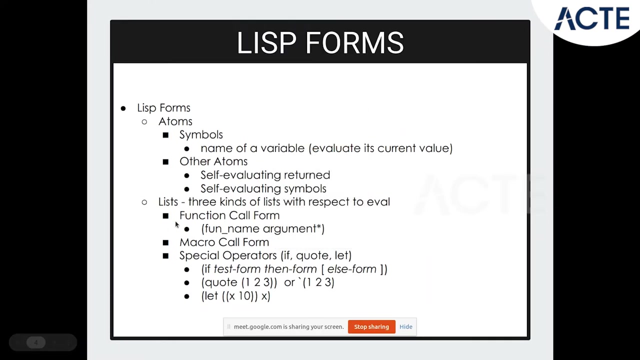 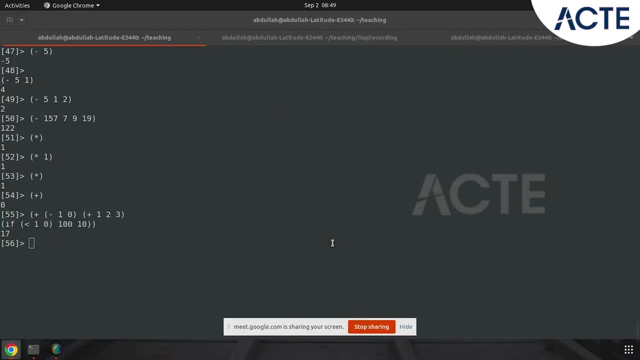 0, so this allows this guy, allows this thing to happen. So what is happening here is basically the arguments for the function name. in general, each argument has to be a valid list form. that is all it requires. So for that example, what we can see: that if you put in an expression, it will not be. 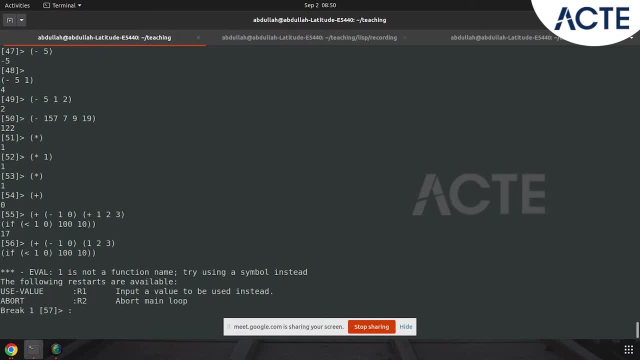 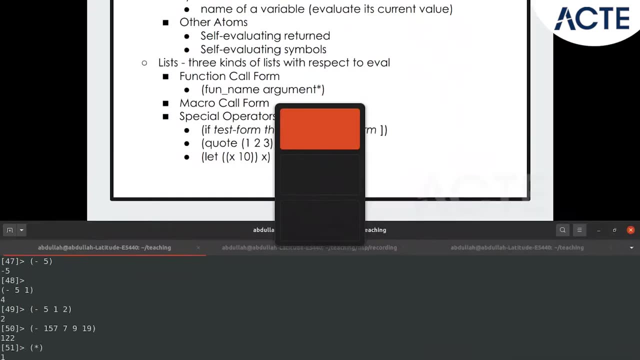 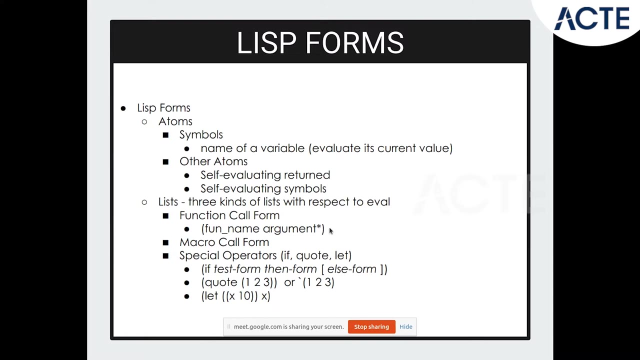 a list form. That is the reason. so it will check that this thing is not a valid list form. So it requires that each of its arguments is a valid list form so that it will evaluate all those arguments. The evaluator has to evaluate all of those arguments. first, evaluate all of them, and 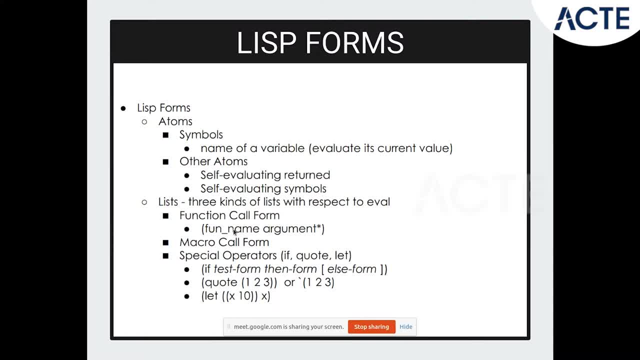 then apply the result of those arguments for this to evaluate this function name. So this is how the functions work in this. this is how they are evaluated. If we can understand this, we can do a lot of things in this. But however, as we saw last time, if is actually a special operator, 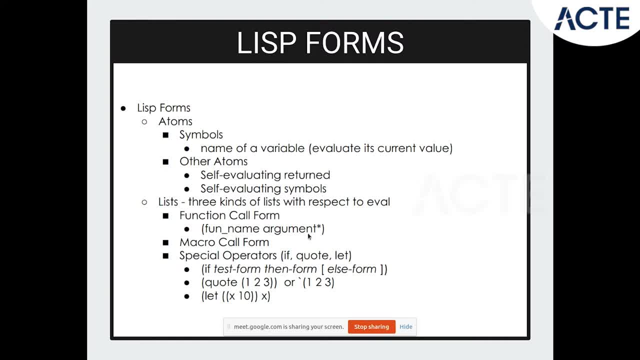 Sometimes this approach of evaluation is not enough, because for the if is a perfect example for that, You have a test form, you have then form and I have an else form. Let us assume you had all three arguments for this if. but if you were to evaluate in? 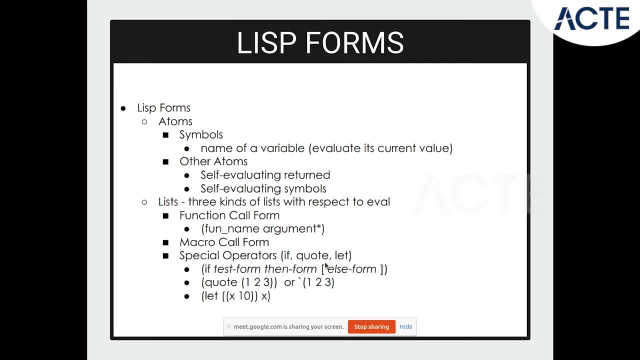 this manner. you will do this, then you will do the inform and then you will do the else form. but then, if you do it that way, if you do it that way, you would end up evaluating both things. but you do not want to do that in this. 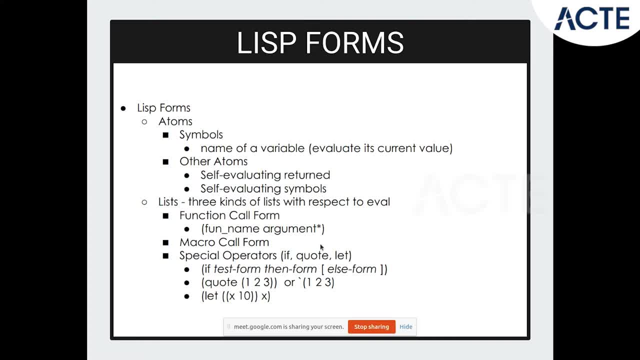 You want to take this and then execute either this or that for that to handle this type of control flow and some for other things also. I mean to some places. you do not. you cannot use it this way. many, most of them is it will. it will suffice most of. 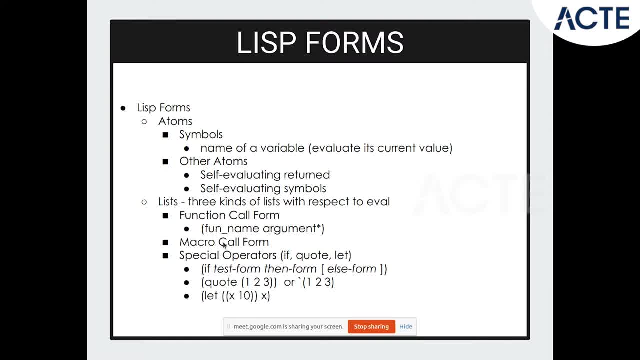 the list programming. It follows this approach, but some places it is not sufficient. So for that you have special operators and special operators. the evaluation will proceed differently for depending on the operator that you use. The three examples I have here: if and code. we covered last time and code is basically: 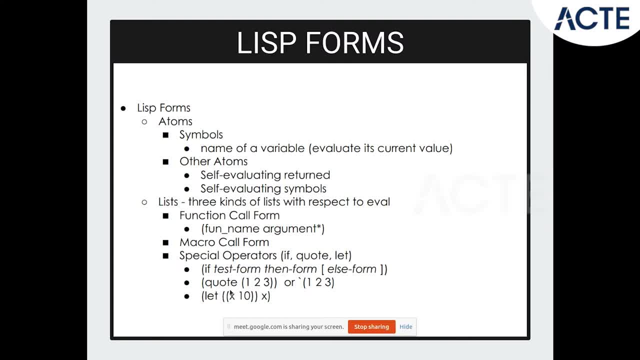 it prevents evaluation. it just prevents you to evaluate it. so it helps you to prevent. so it restricts the evaluator from evaluating that thing. It says: just evaluate. Just use it as it is. do not evaluate this part, because it protects the arguments from. 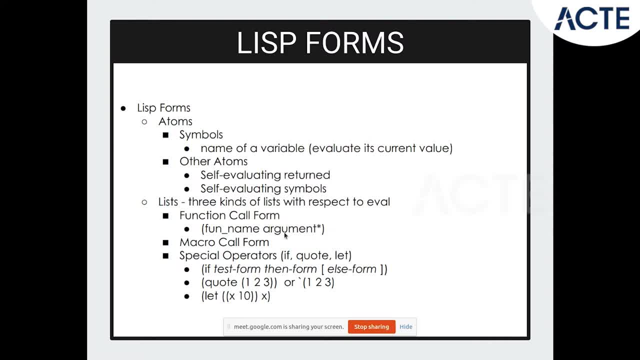 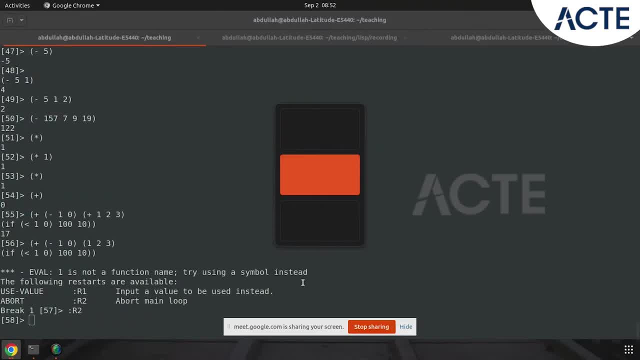 getting evaluated so that you can just use it as it is. So there are some many places where it will be useful- and we will see examples of that And this instead of code code- and there are many places where you will have shortcuts. 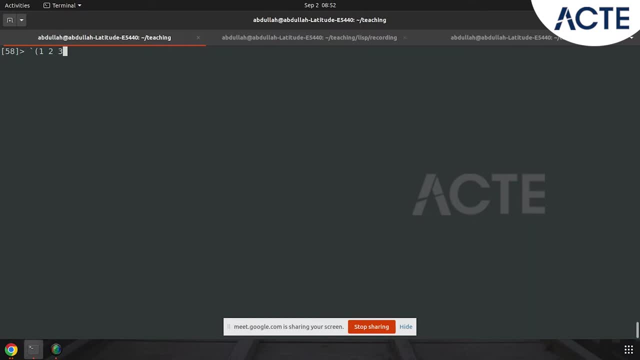 This is a kind of a syntactic sugar for doing code. You can see this. You can see that you can use equal and ask whether 0u over p of 1, this will be basically the same thing. That is it. 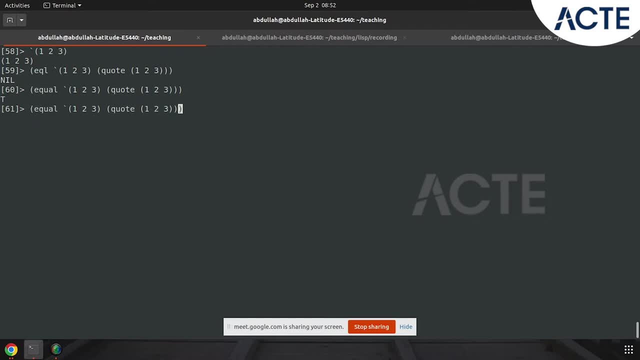 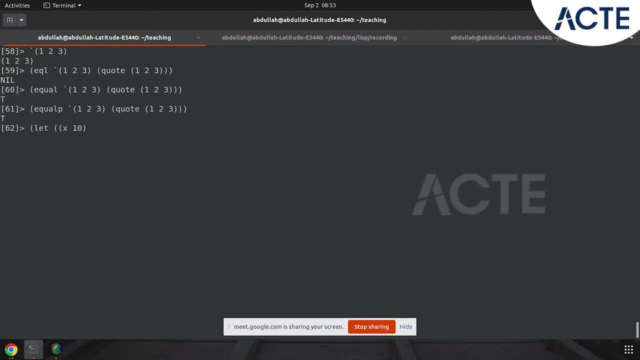 Thank you, And let let is another construct. So what let does, is it? basically it defines. it allows you to define one mistake. It sets up the environment. So let allows you to set up an environment where you can specify some arbitrary things. 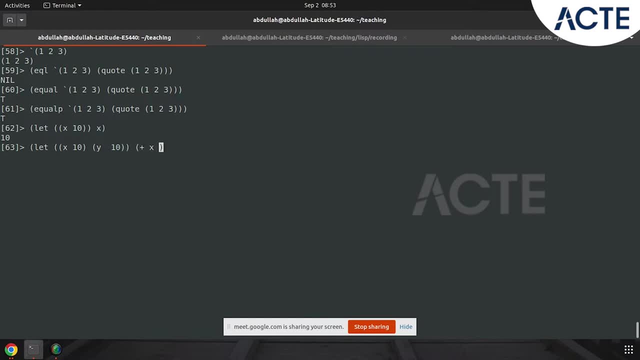 I mean you can specify: okay, I want this. it modifies the environment. So the, even your yes, when you so let construct is like it starts with a let. So you can see that we do not use it. it is not considered to be a function form because we cannot have this by itself. 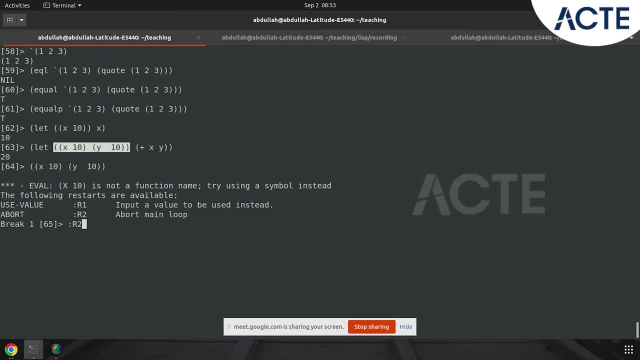 This is not a function name, This is not a function form. So let what it does is. it basically takes this x and 10 and it modifies the environment, So it is like a side effect. So whatever is inside that, let first. the first part will be the sequence it will be. 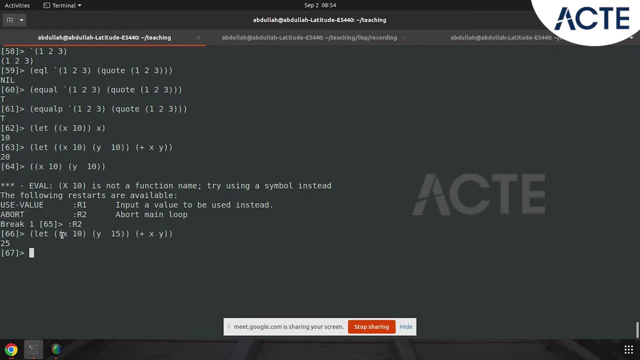 of this form. It will be a list where each list item is a variable followed by its value. So you add all of this stuff and you can have arbitrary number of variables in the first list, And the second list will be where you can write arbitrary code. So this is. 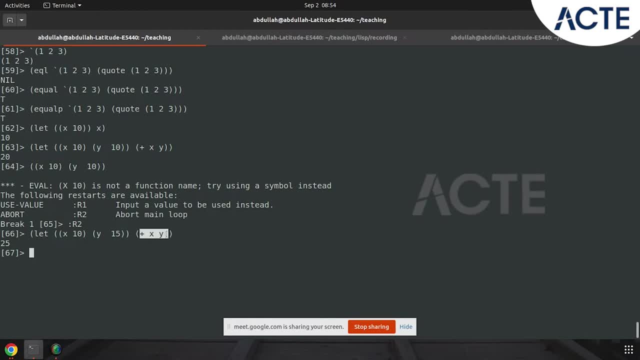 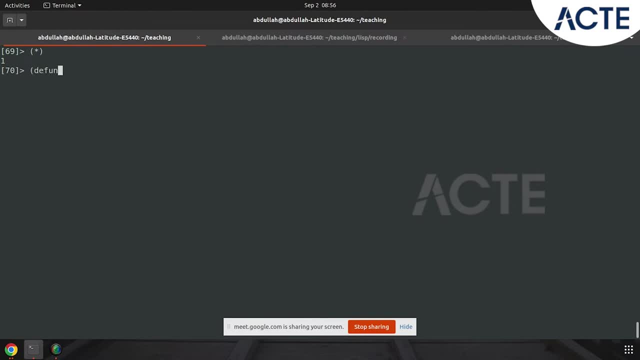 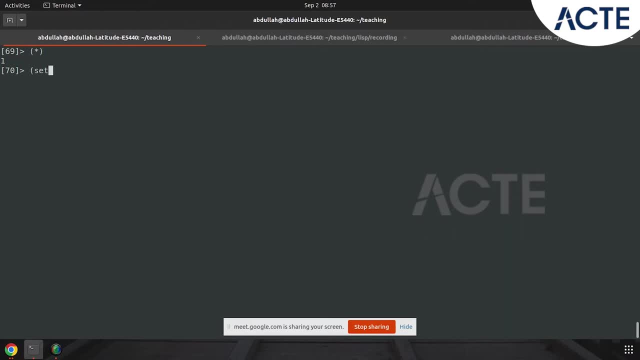 let us set, let us put it as, like, say, 100. all right. now I am saying, if let us see mod of mod x 2, that is undefined. okay, mod is basically a thing. okay, mod 3: right, I hope this is clear. mod 3 is basically saying that, okay, whether it is even or not, okay, okay. so mod 3 says: 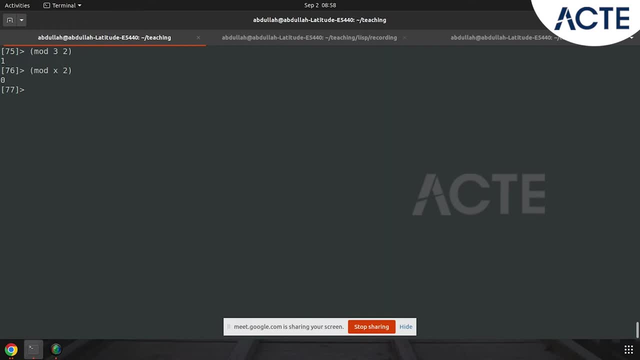 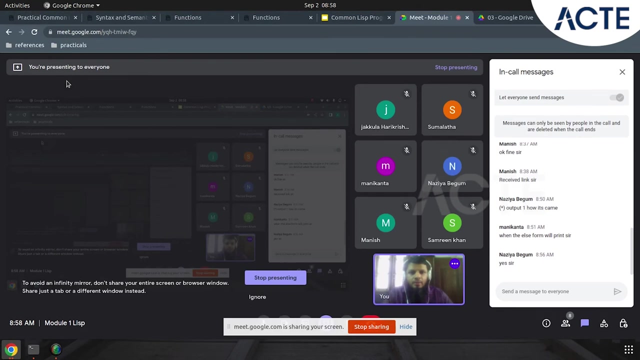 whether that thing is, that number is even or not. So mod x 2 will basically define evenness. now if I say: if mod x 2, let me define a function, yeah, so define. okay, I am giving, I am introducing the next slide. okay, so the next slide, we. 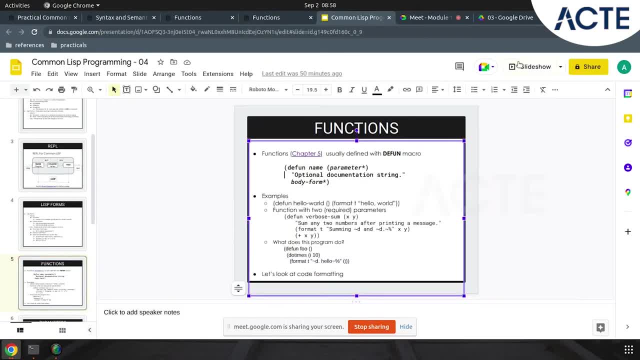 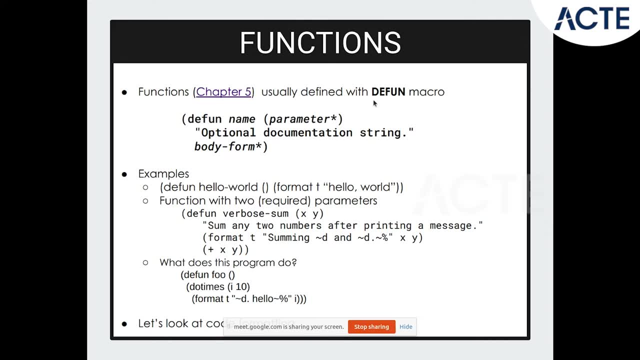 have what? let us introduce the next slide and do the same. do the same, So define. this is how you define a function. okay, Let us see. So the note that define is a macro, macro form. we will not get into macros right now. 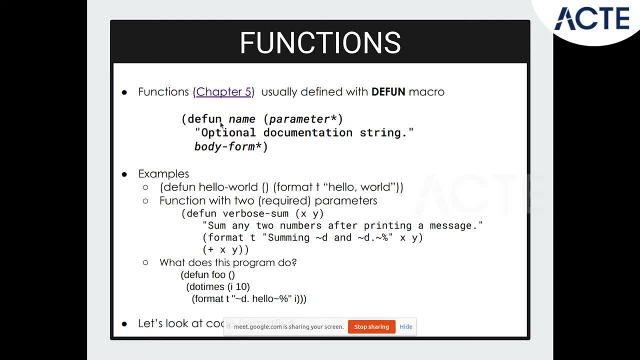 but it is similar to a function. okay. only thing that this is not the name of a function. it is something else. we will come to what that is later on. but this is a macro. okay, and the macro condition is only the first thing. the name will be a macro name, but rest. 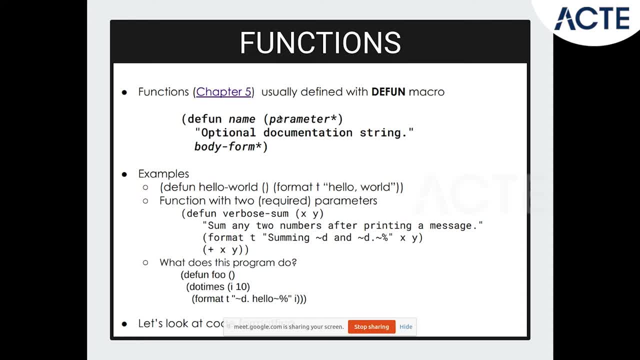 of the things. it has to be an asset. asset, as usual. okay, macros have this thing, so we have the macros, but basically this is a macro name and the rest of the thing for defining the function. you have to give the name, you have to give the parameter star, so you have. 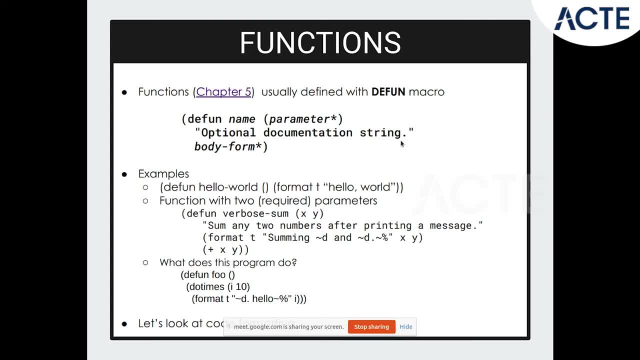 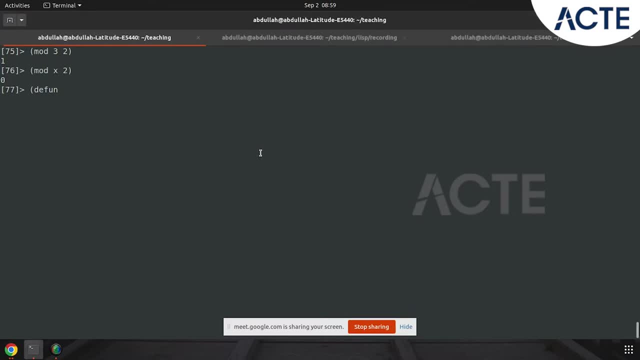 to open the list again, you have to do a parameter star. you can have a string, literal, and then you can have a body form, clear. this is how you define a function. so let me define a function now. define function like: Okay, Now, this is come, this letter. yeah, this thing comes okay. 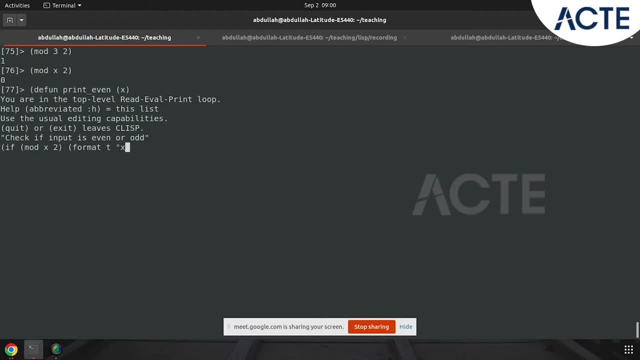 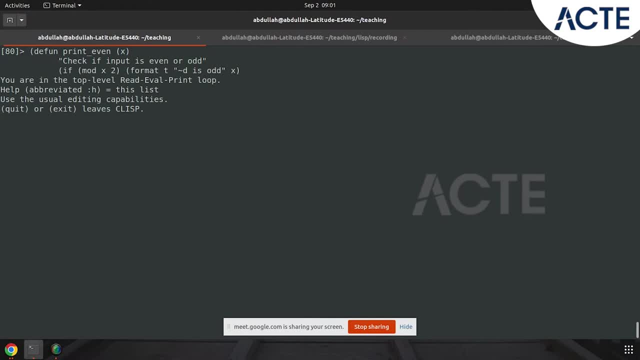 I am also using the. I am trying to explain how if works also, So while explaining the different functions. so basically, we can do both things at the same time and see how it works. This is how the function looks like. Do you understand how it is working? 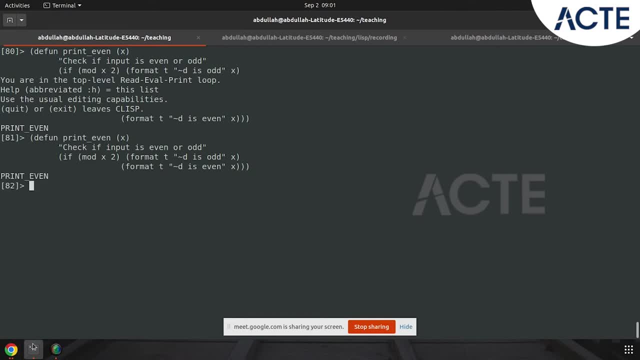 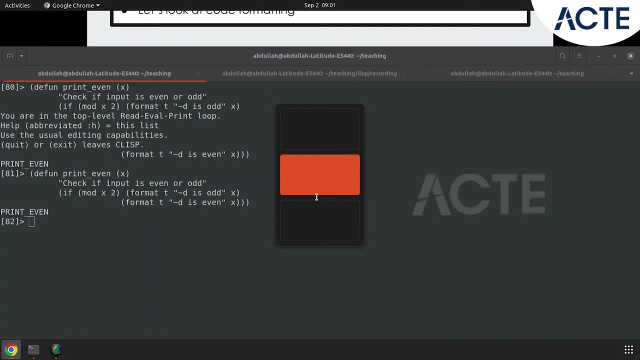 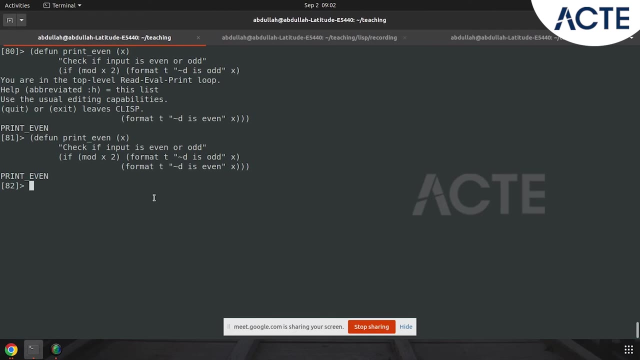 So did everybody get the definition of function? Maybe we can go through the definition again and come to the if thing, how it is working. So let us take a simpler example. So let us continue with the example. So let us go with the first. let us do the hello valeta example. 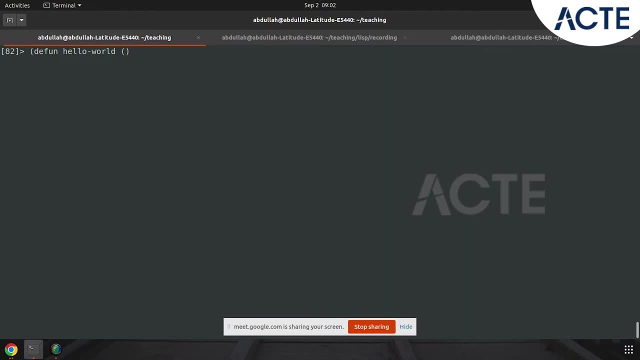 You are getting comfortable with the definition of a function. So this is: you are getting into the function definition which is like, which is like pretty substantial amount of list. If you can just get the functions going, you understand how the functions work. it will. 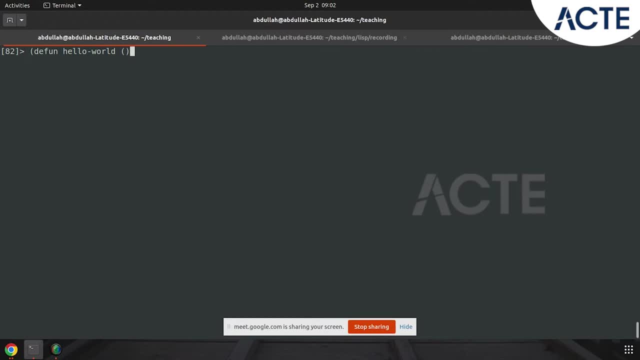 help you to do a lot of stuff and just do a lot of things and list, But some things you might you do need special operators and macros. macros are really very good support Okay. So even if you do not write macros, you still have to understand how others have written. 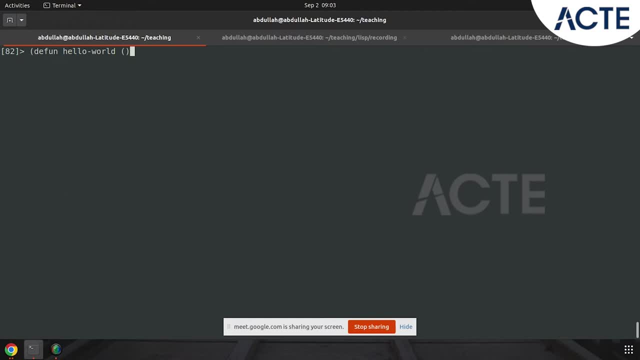 if you go through a library, right, somebody would have written macros and you may need to understand it. So it is necessary to understand all of it. But the difficulty, if you can get through the function calls, if you can understand that and do that well, you know. understand that you more or less can do the other things. 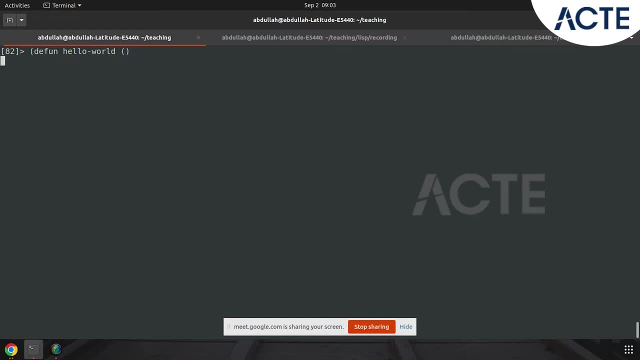 also All right. So this is how the function call looks like. Okay, So this is actually an invalid form. get it. So what happens is the body, this is the. I think this is the function name. these are the parameters. 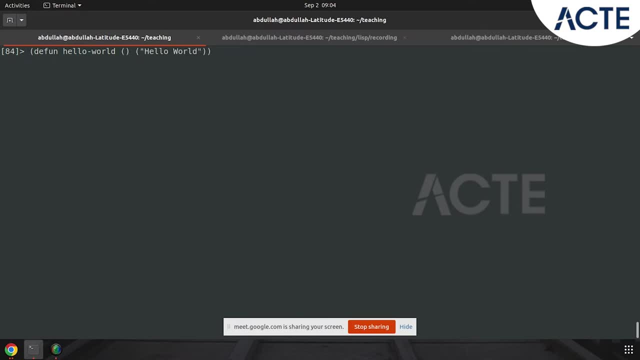 Okay, It parameters that have to have a. it has to be a list, So it has to have open index. It has to be a list. Okay, It has to be in a closed place. It could be empty. This is what we have here. 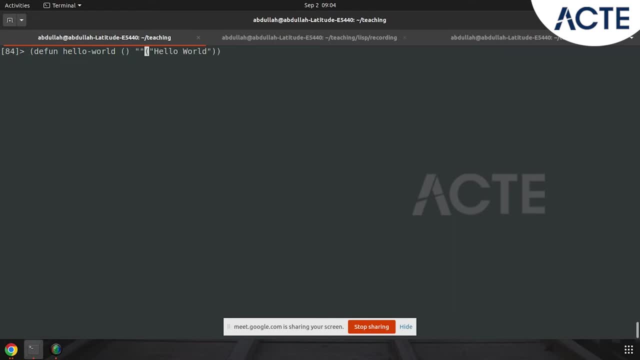 We do not have any input here, And then what we can have is we can have a string which could be empty, which could be it is optional. Okay, You do not have to put it there, but if you put it, it will give you a documentation. 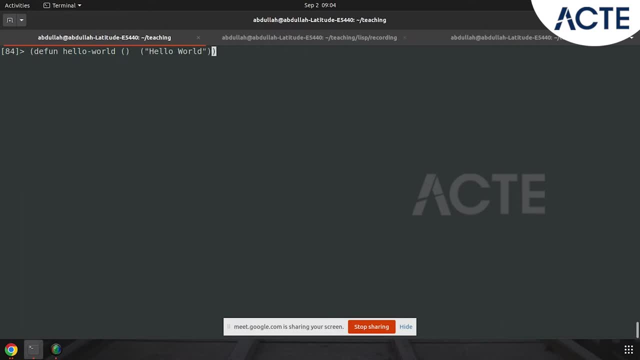 Okay So, but this, this part, this has to be a valid S expression. Not only does it have to be a valid expression, it has to be a valid list form. Okay, So, for making it a valid list form, I need to do something like this: 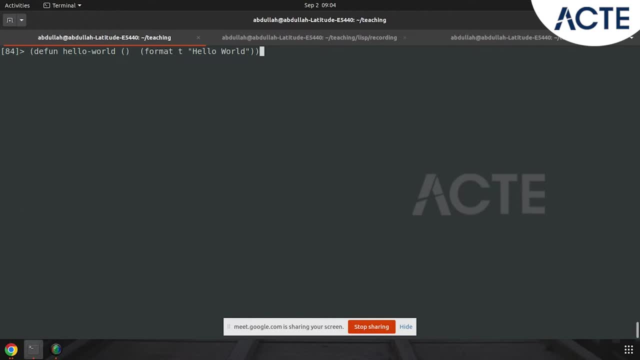 Is it clear. So my function is defined. now, All right, If I say hello world, I will get the output Clear. So we are getting into interesting, interesting territory. So this is like the core of list. So, if you can, you have to, you know, be able to work with functions and more or less it. 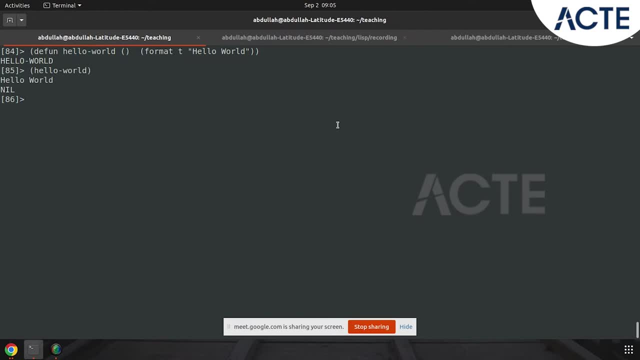 will. yeah, it will. basically, you are going to start doing some interesting things, Okay, And it also, in order to do it properly, you need to recap and recall all the fact that we- I mean all the concepts that we have understood so far with respect to S expressions. 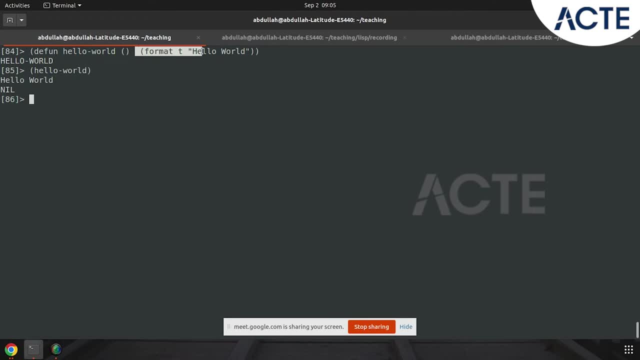 and list forms. So, for example, here I cannot have, we cannot have anything. even if it is an S expression, it is not enough, It has to be a list form, All right. So this is something you have to take note of. 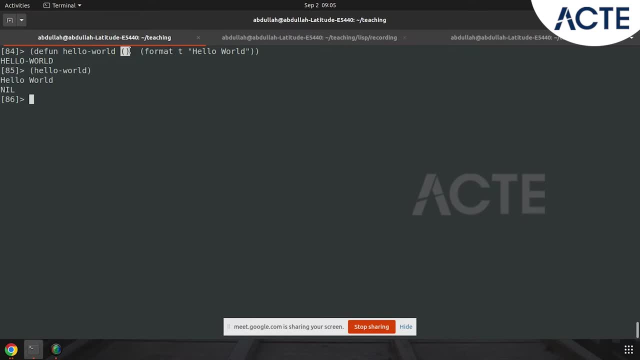 This thing has to be a list form. This is a list of parameters. We have an optional thing here And you can define functions like this, Coming to the if thing that I had said. So let me just go back to if. Okay. 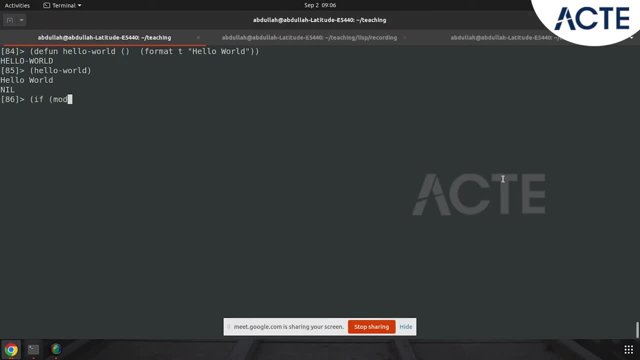 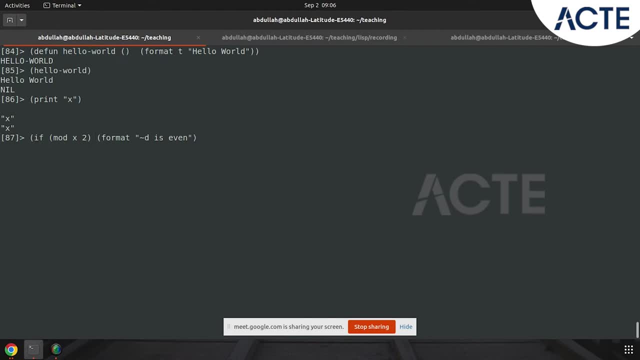 What? Okay, Thank you for that. Okay, Okay, Thank you for that. You don't need to. You can come back to that in a minute, But in fact, you know, I don't think it's going to work. 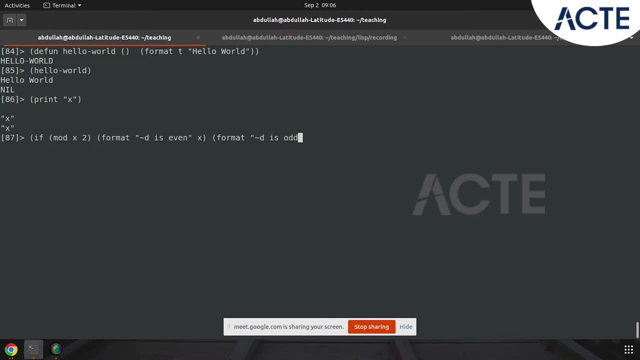 But let's see what format it is. Okay, So 100 is even. do you understand this Manish, how it is happening? Yeah, so here, what happened is this is the condition that was checked. So, though this looks like this is an H expression, this whole thing is an H expression. 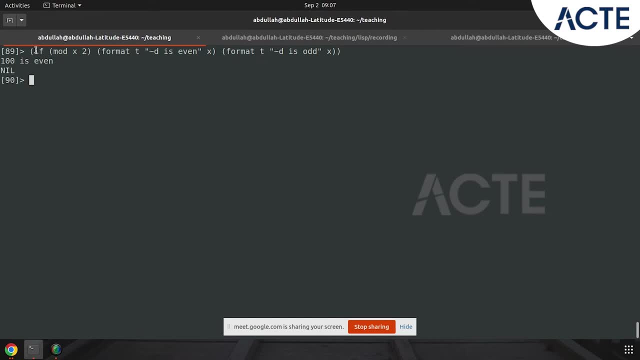 But it is not a. if it was a function call, what would have happened? This has to be a function name first, And it so happens that if is not actually a function name, because it is predefined, it is a special operator. 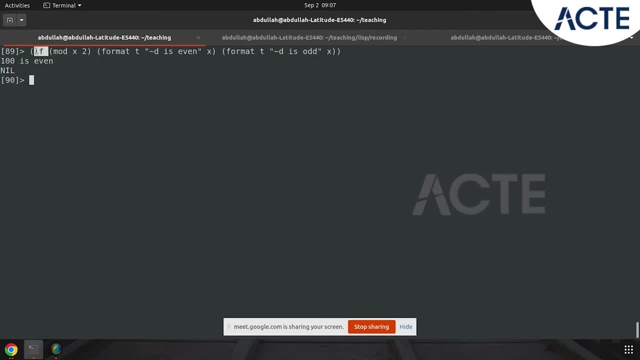 So there is some thing for in list you will have some special names. special keywords are there. if is actually a keyword, So it does not take it as a. it does not treat it as a function name, first thing. So it treats it as a special operator. 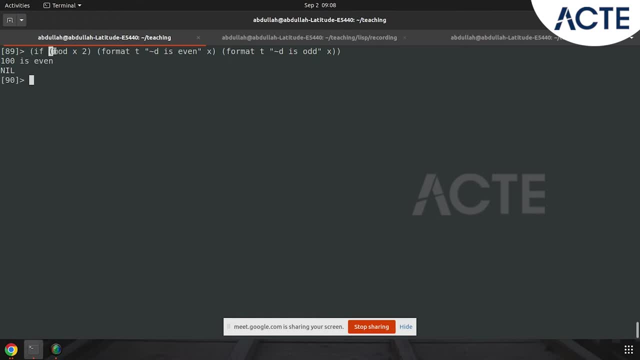 If it were a function name, what would have? what would have done? would have evaluated this thing And then you will get a result. Let us say: this is has to be a has to be a Boolean result: true or nil. 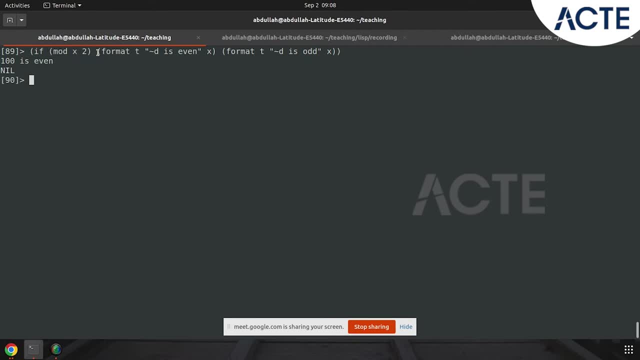 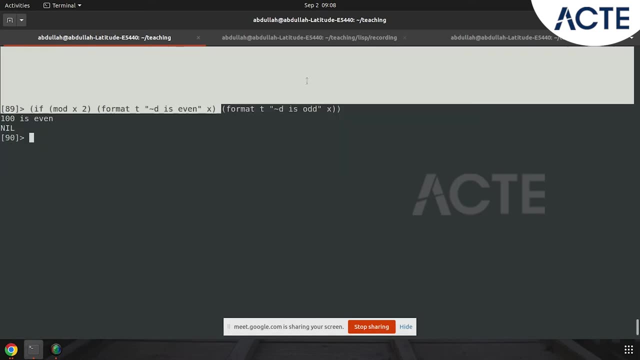 It would have evaluated it. But function call. what does it say? you have to evaluate all your arguments, So you would have to evaluate this, then you have to evaluate this, But by the time you do that it is gone. I mean because then you have to evaluate it. 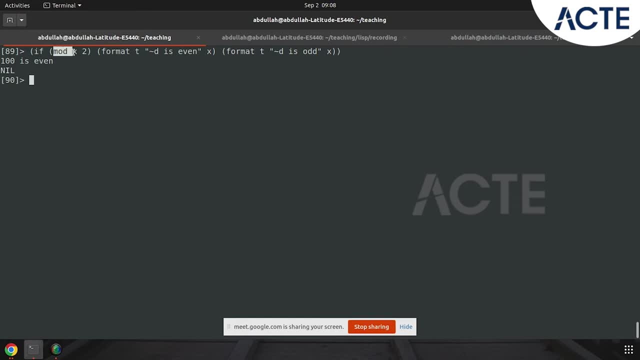 But the point of it is to execute based on the result of this. So the control flow has to be regulated based on the result of this. If this is true, you do this, And if that is false, you do this. You cannot implement it. 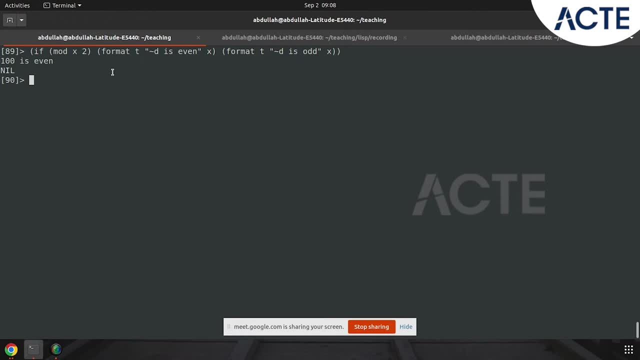 If it was false, you do this. If it was a as a function call. that is the whole point. I am saying So. if that is why, if is a special operator, It is also a list form. list form: it is a list form, but it is a special operator, not. 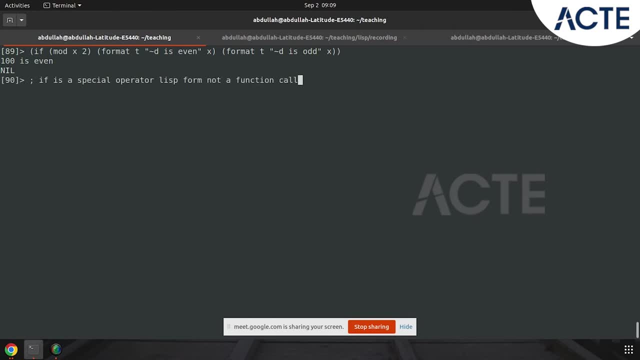 a function call. This is what I wanted to say, because function call is uniform. You give a function name, Then you give argument 1.. Depending on how many of our arguments it is accepting- And some- it could be variable M. So there is a lot of flexibility here. 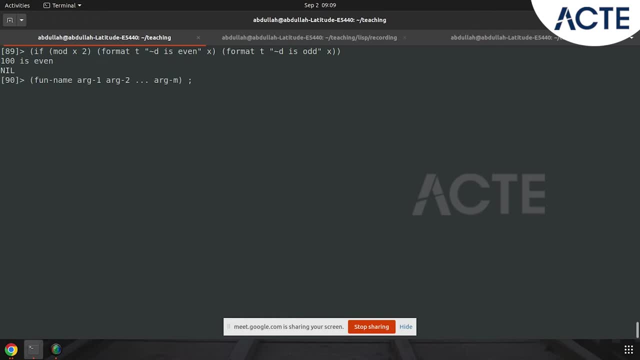 We will come to the function call arguments. But if it is a function call, every arg i has to be a list form. It need not be a function call. That is the thing. It has to be a list form. It has to be an x expression. 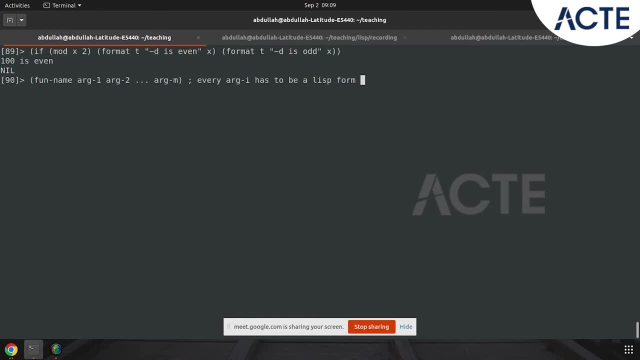 And it has to be a list form. Okay, It need not be a function call. It could be a function call. it could be a- this thing, It could be a, it could be a function call or it could be some other list form. 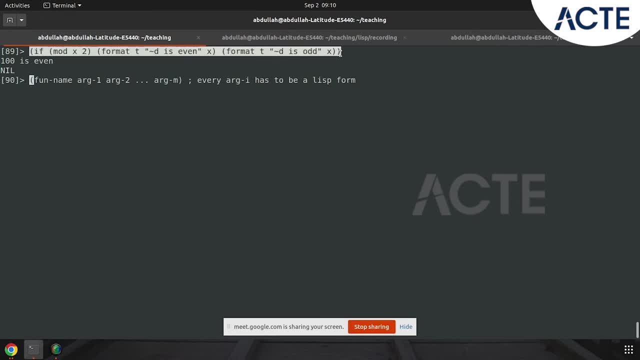 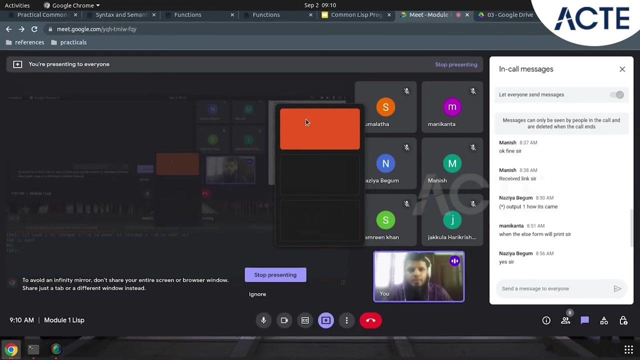 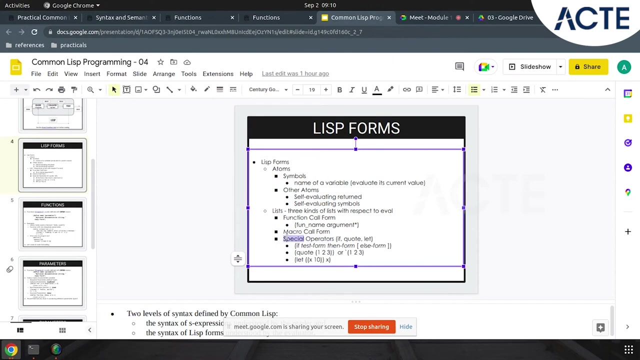 It could be something like this: You have to get the recursive decision very clear. It has to be a list form. I hope that is clear now. So now, and if is a function, if is a special operator, Operator, what do you call it? special list form or it is a special operator? 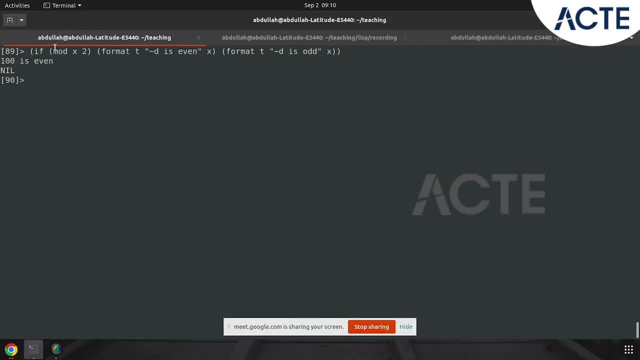 It is a special operator form. Okay, So that we will evaluate, based on the, on the definition of, if It will behave like a if operator. Okay, So it is all about combining things, So it is very easy to see, one by one. 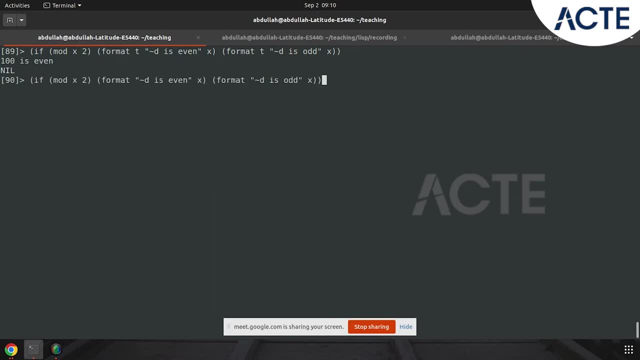 Okay. The difficulty is when you combine the things to create something like this: okay, to create a functionality. So you have to be very clear on that and you know, see how it is, you know getting combined and how you are writing it out. 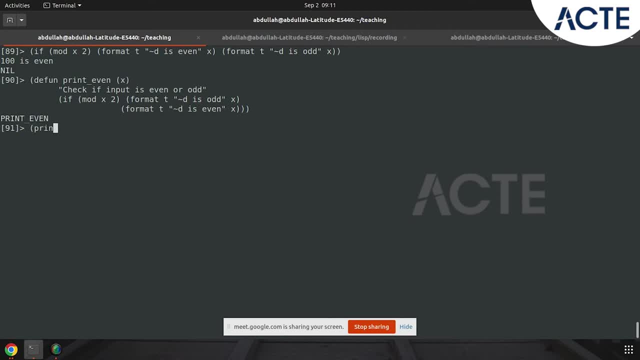 So we will again. this is all about you have to do a lot of exercises for that. And another thing is convention is that you do not have underscore. Okay, You always do hyphen, for you know defining things: Snake case and all that. 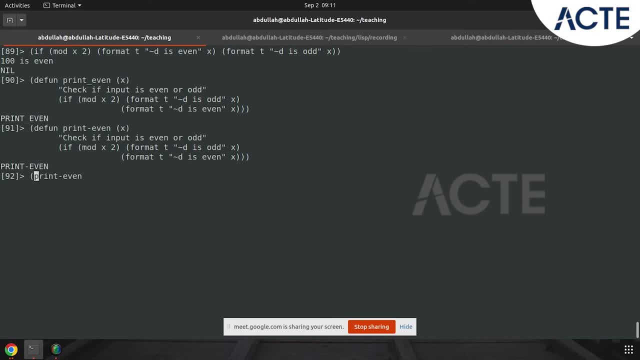 Snake case, camel case is not useful here. All of it is. All of it is hyphenated, usually because it allows you to hyphenate, So print even 100. Okay, So basically what happens is again, if you see, this has to be a list form, it need not. 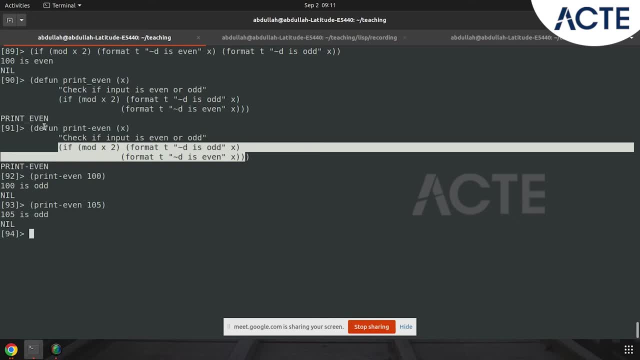 be a function form. Okay. So the function definition of function says: you give me your name, give me some parameters. Okay, Tell me how many parameters you will have And if you want, you can give the documentation, and if you don't want, you don't have to give. 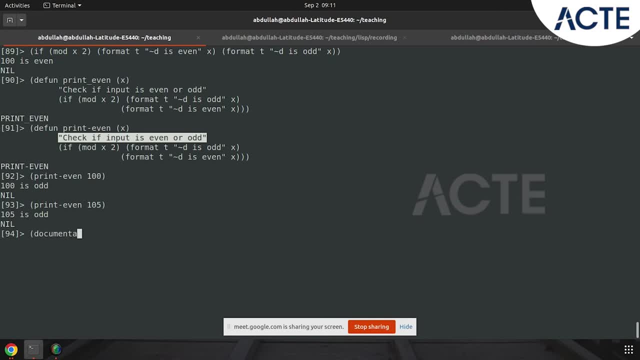 Okay, But if you give a documentation, you can always get the documentation out like this: Yeah, It will print out the documentation, So it's like a help thing. Let's see if this thing works Right. It doesn't have a documentation. 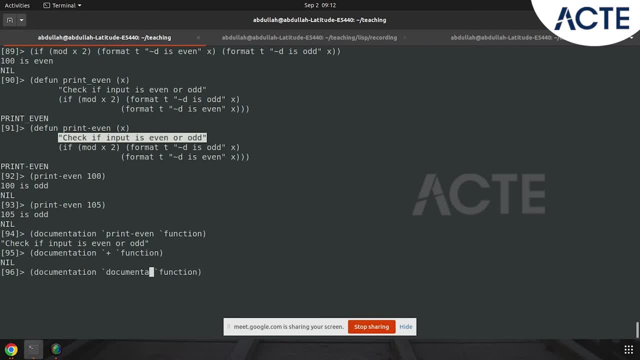 Yeah, But yeah, So if you have a documentation, you can print it out like this: Okay, Yeah, Okay. So if you have some libraries that you're importing, you can actually write down this and you can get the documentation out of it. 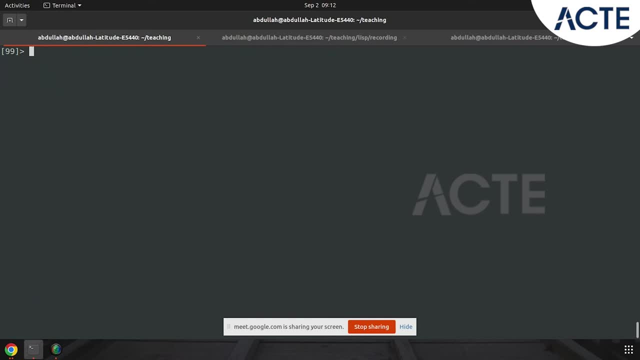 So these basic functions don't have much documentation. So, and there are some, there are some guidelines on how to write documentation and then not only So we can look at that, but that's basically how documentation, I mean, how the function. 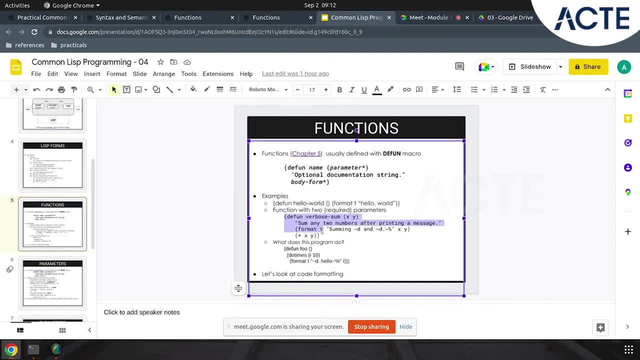 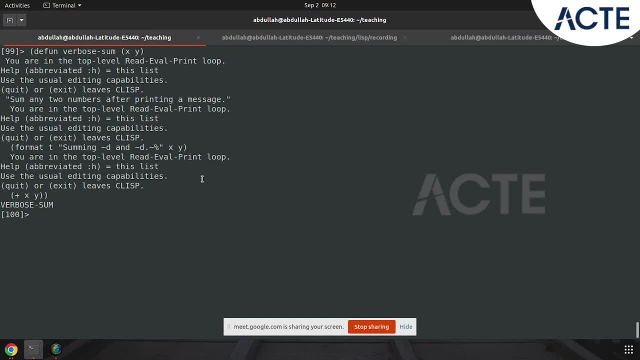 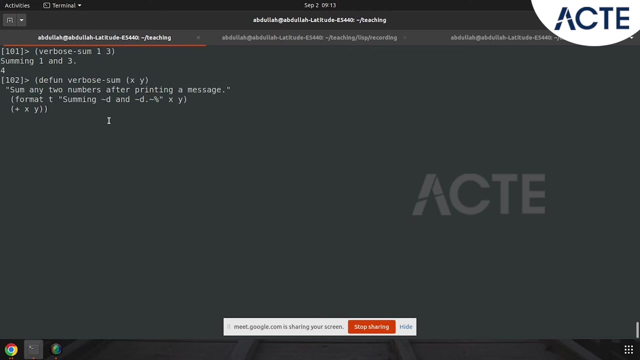 is defined, Okay. So let's take a look at this thing. Example: Yeah, Yeah, Okay, Yeah, This is how I think function is defined, So you can see that you know format t and plus x, y. 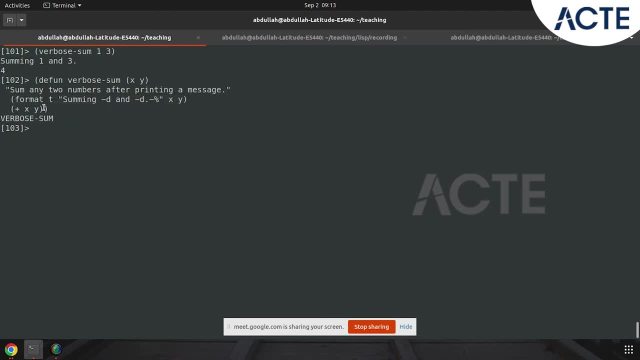 So it can. it is a series of expressions. they do not be just. you know, it is a list of s expressions, So first this, then you do this, and so on, So you can actually define things like this And the result of that thing will be the result of evaluating the last s expression. 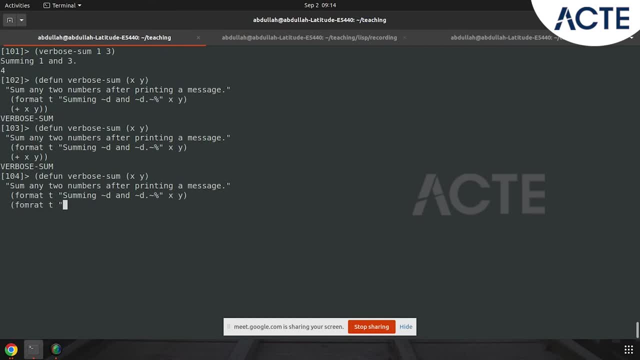 Let us take this. So this is the last expression. It is s y n, So we have y n y n, So s y n y n. And then this other one is as follows: 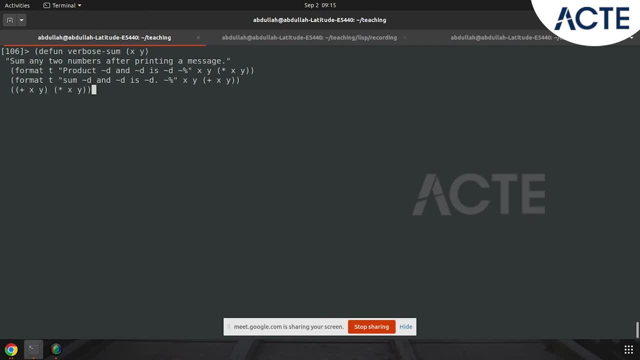 So this is the last expression. Let us take this, So you can see that. so this is the last expression. This is the last expression. So this is the last expression. okay, so it's defined. now maybe I should not make it, yeah. 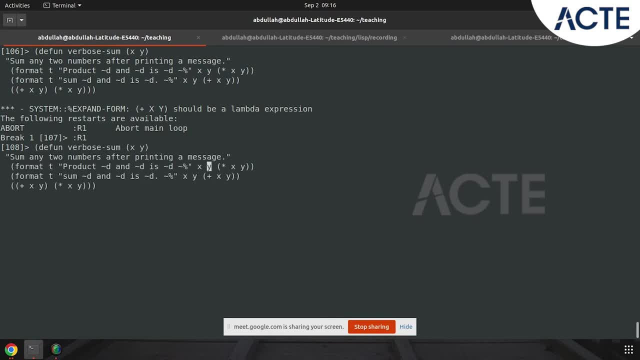 you have to make it a verbal and I think you need to quote it. yeah, doesn't make sense, okay, so sorry. yeah, you can make it a list here, so just keep it simple. this is the definition, right? can anyone explain this? do you want to explain? okay, sorry. so what are you gonna do it? you already actually. yeah, so what is this? 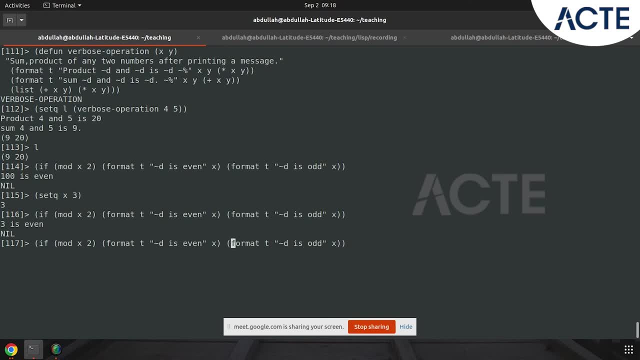 it's basically a void x. two is, even though it's a, after what he'll do it, you have to do this. equal in it, equal to write 0, so that's try to enable this to. what happens is mod 100 to is 0, mod pi 2 is also 1.. This is actually both of them are. 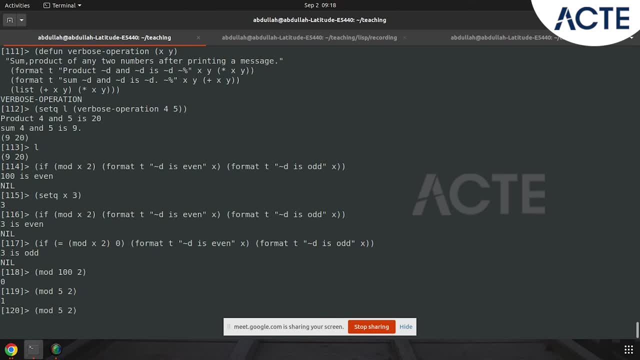 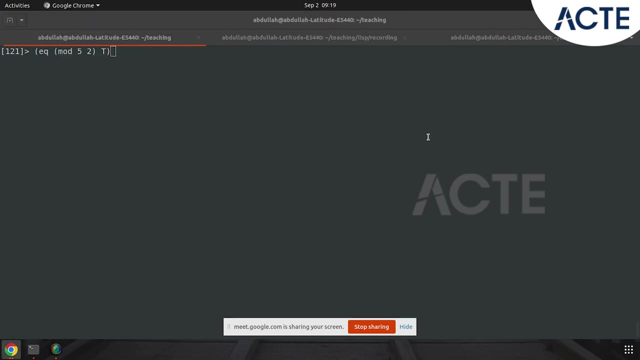 considered to be true In Lisp. anything that is not nil is true. That is the issue here. This is actually. true, is always true and nil is always false. But anything depends on the operators: how they deal with the non t and non nil. So it so happens that this is actually. 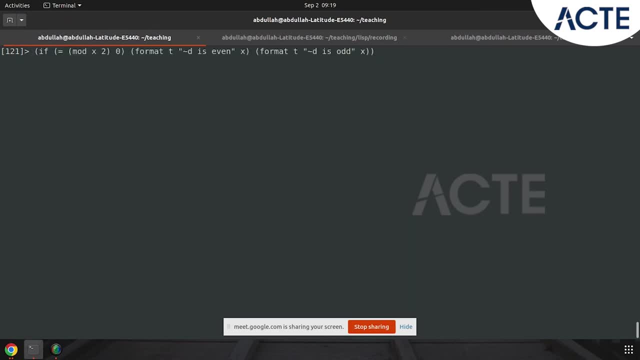 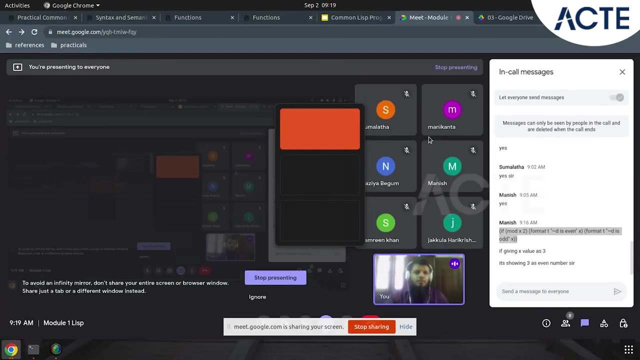 something which treats anything that is not nil as true. So that is why it always does that, this thing. If you had the thing here. so what do you want actually? is that if mod x 2. And it should be equal to 0,, then it is even otherwise. it is odd. That is how you implement. 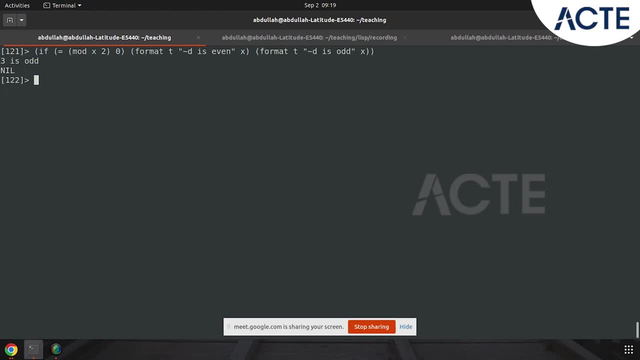 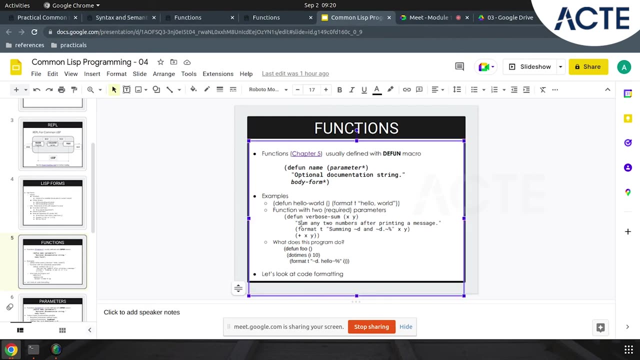 it. So now we are defined, So before. so let me just complete the rest of the thing. let me just give you an overview of what we can do with this. So let us just go ahead with that. before I give you the practice, I will give it an exercise. 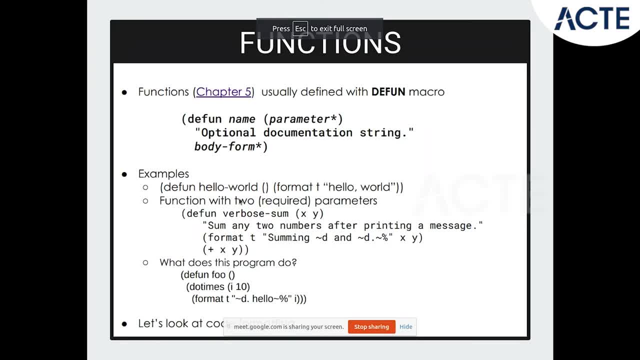 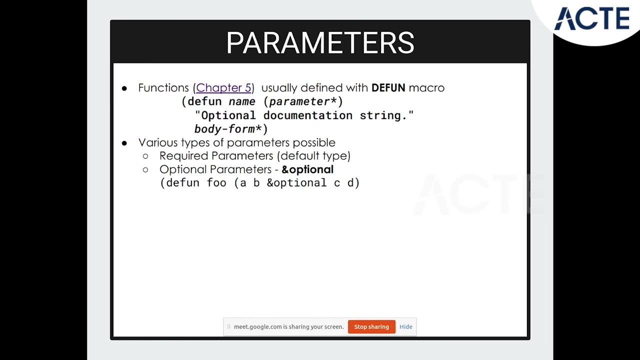 So let us just complete this thing as a project. So, as you saw here, this x and y are both required. This also give it as an exercise. and the parameters: there is a default parameter, there is a rest parameter and a keyword parameter. 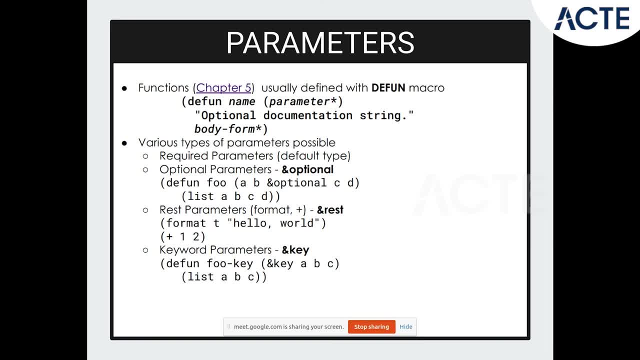 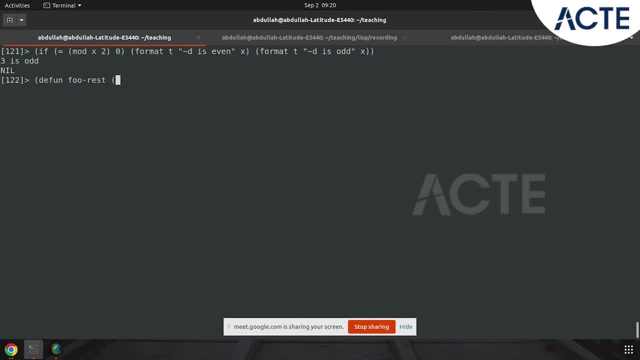 There are different types of parameters for a list. So, for example, we saw this: whoRest, AmazonRest values. So, just as we saw the, we saw this star has multiple values. So how do we do this? You can take 1,, you can take 2,, 3,, you can take 4, it takes an arbitrary number of arguments. 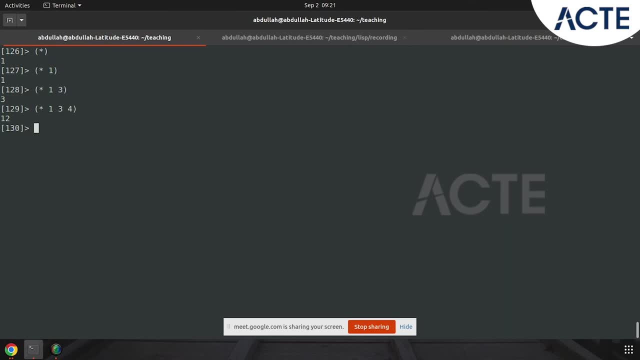 It does not take, just it is not. well, it is not like 2, 3 arguments. it can take arbitrary number of arguments To do that. how do you do it? You have something called the REST, And this is how you do it. 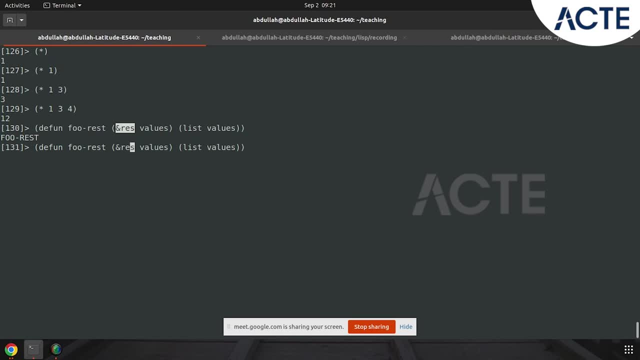 So there is a REST. sorry, it is a REST value. So whoRest it is a nil. by default, it will be nil, but it will have, like you have, 3, you can do this. Is it clear? 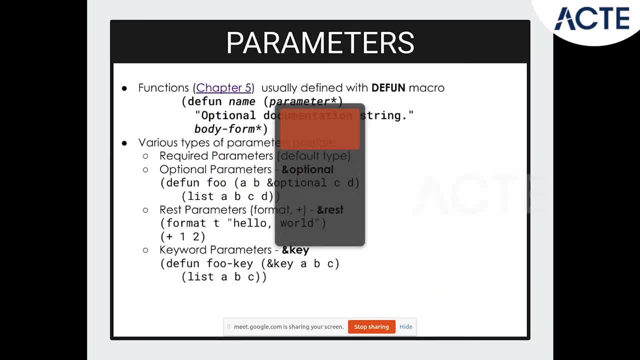 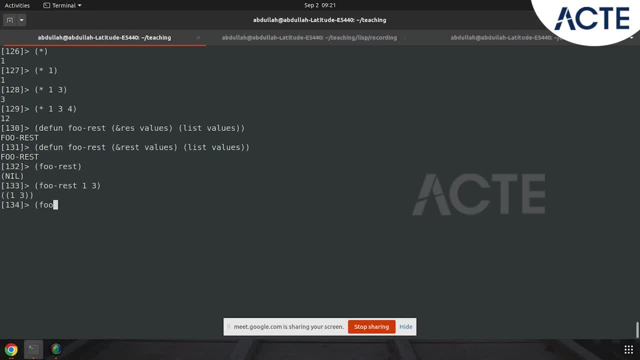 What is going on here? It basically catches all the. it allows you to specify things. but even simpler than that, it is this: optional: Okay For optional, and let us okay a, b, f, c. Will this thing work? 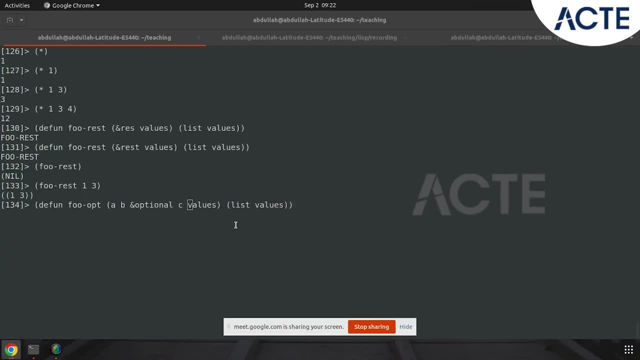 Yes, We can do it. Let us do it. Okay thing work. okay, let's see. let's go back to previous thing. of course, some six gives you, so this will not work because it requires two arguments. okay, this will not have too few arguments: zero instead of at least two. so notice that. 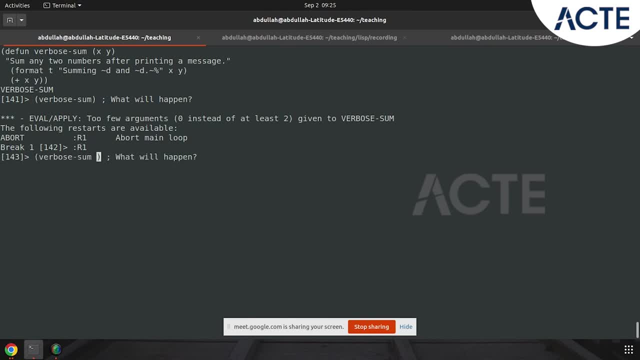 it's saying at least two. okay, so you should give, like uh, one, one, one argument, not two. you have to give two arguments, okay, so this is the default way of uh getting parameters. all right, these are all default. these are. these are called required parameters. these are required. 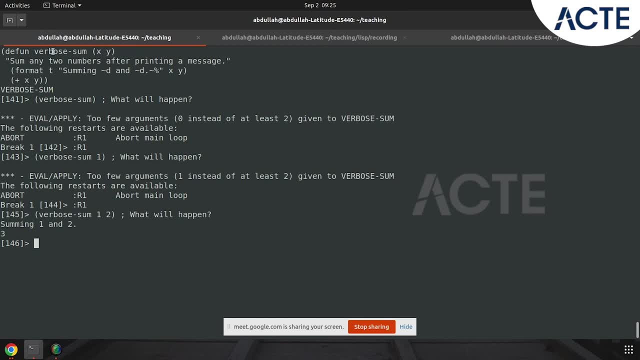 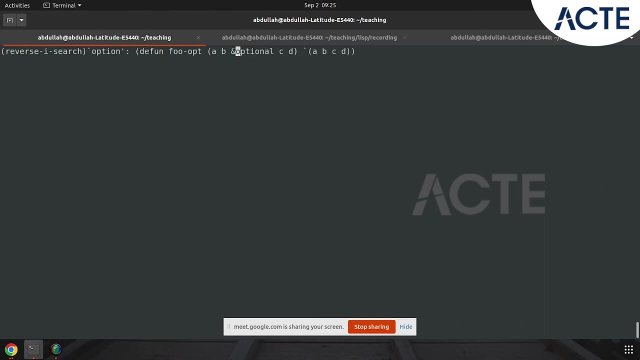 for you to even call the function. if you want to call this function, you have to give this x and y, otherwise you have to give two values and then only you can call it all right, otherwise it will not call. whereas, uh, for optional you. yeah, so i can define a function and it can take optional values. 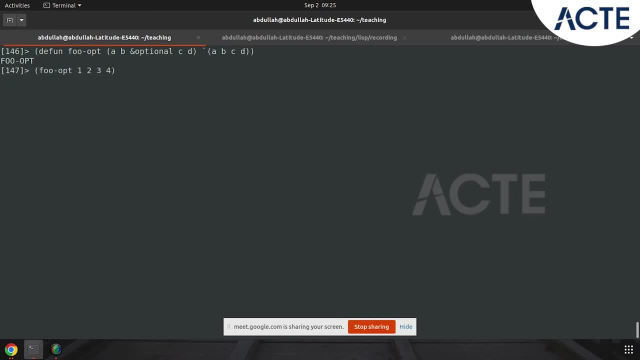 will this work? it does, okay, so you get the values here. will this work? so, basically, it depends on what this optional does, okay. so what optional does is, if you have to define optional and the thing that follows it, it will be optional, right. so this option cd. 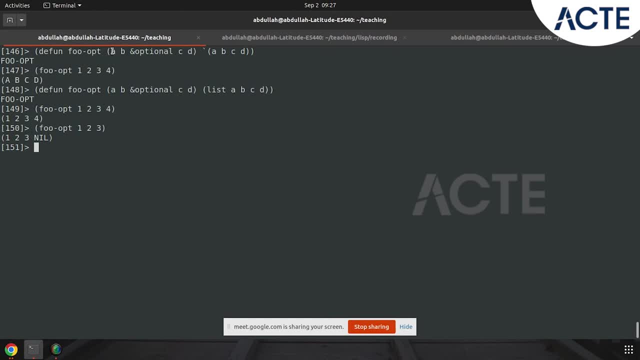 so what happens is uh, so, uh, required, required is like a and b. okay, this will also run, gonna be functional. um, i know the thing is that like chemical, natürlich, okay, okay, can it will, this will also run. so, okay, this will not run. okay, because you need to al buat. 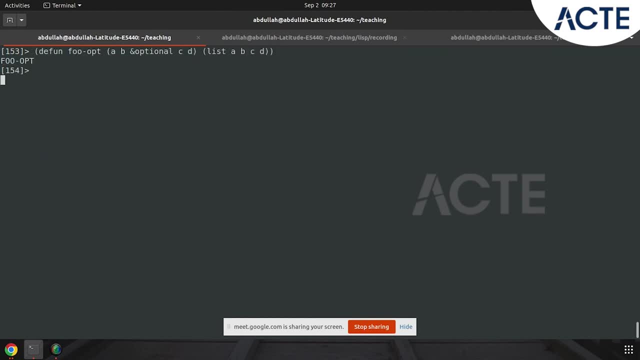 okay, this will not run. okay, because you need to see that. okay, so this will be an option. it should not just play verso after this. okay, this will also run some such. okay, this will not run. okay, because you need to see if this is necessary. you need at least two arguments for foo opt. so for foo opt, you need at least two arguments. 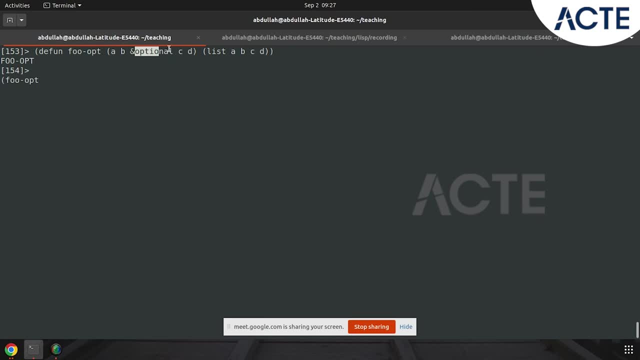 so the things that, uh, optional. how it happens is you write optional and everything after optional will be: either if you want, you can include it, or if you don't want it, it's optional. so those are, those arguments will be optional. okay, so one, two, i can have a function just like this: 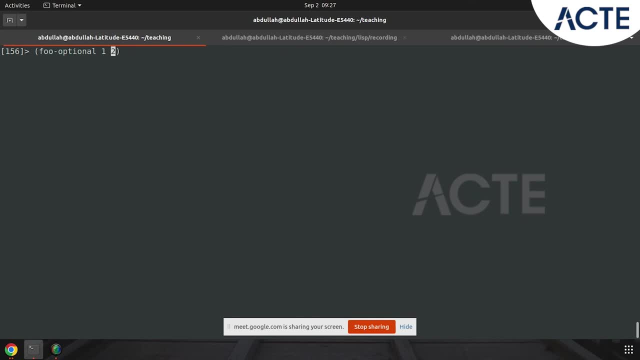 let me see that go out. i can have a function just like this. okay, i can call the function, because a and b are without specifying anything. they are keyword parameters, okay, so i have to specify, i have to use, uh, specify values for that. but what is that if it is? 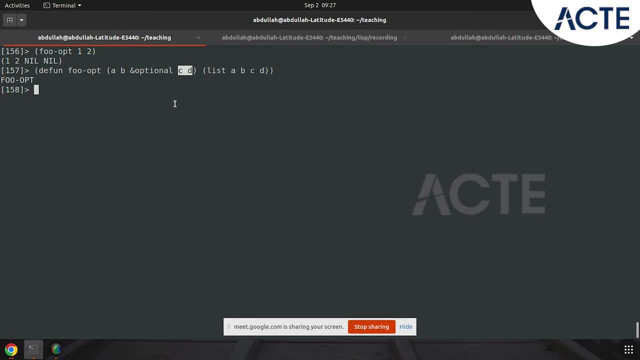 optional. anything after optional will be optional if you want to include it. if you don't want, you don't include it. and in fact, what you can do is you can also have default value, see how hundred? okay, and this default value will be what it takes up. you don't specify it, but if you say 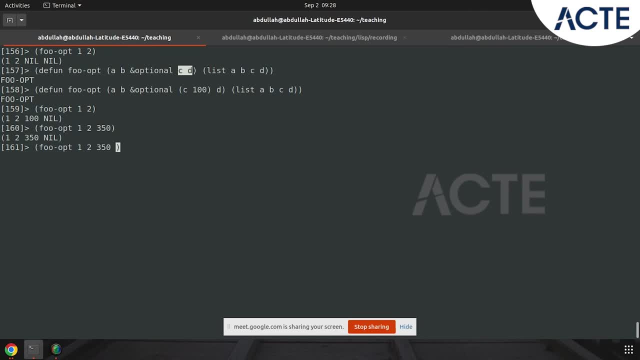 let's say 350, it will take up that 350.. if you want to say 1500, it'll take up. so optional, basically, what happens is, if you want to specify it, if you don't want to drop it, this is what optional doesn't okay. but however, what happens with optional is: it's good, you can define. but 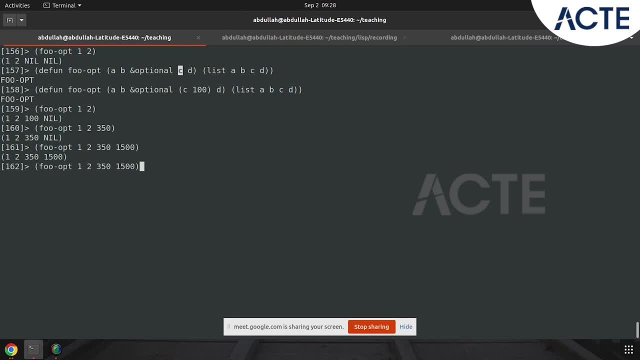 you have to. it's discrete, so you can. you have to specify a upfront. i cannot have like arbitrary, all right, there's too many arguments. so what this function does is that it accepts. it accepts at least. it needs at least two things that have not been defined with uh. 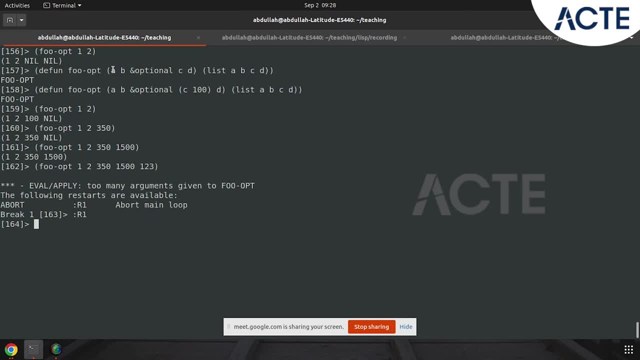 which have not, do not have any qualifier before it, uh, which are just, you know, named as variables, as symbols. they have to be specified. so you cannot have one, you have to have at least two. you cannot call it without any arguments, you cannot call it without arguments. you have to specify at least one, two values, you cannot do one. 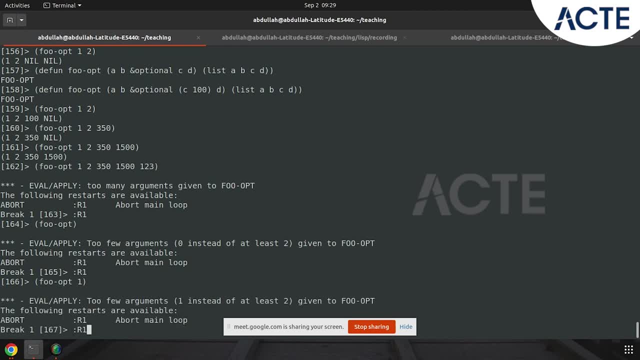 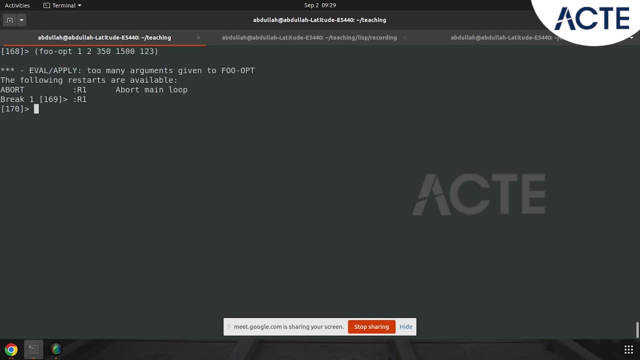 also. so you need to have two values. but uh, yeah, yeah, you can. you have to have two values at least. so you have to have two values and you can go maximum of two. so you have to have two values and you can go maximum of two. you can specify default values. so what happened here is: uh, you know, the c is 100. 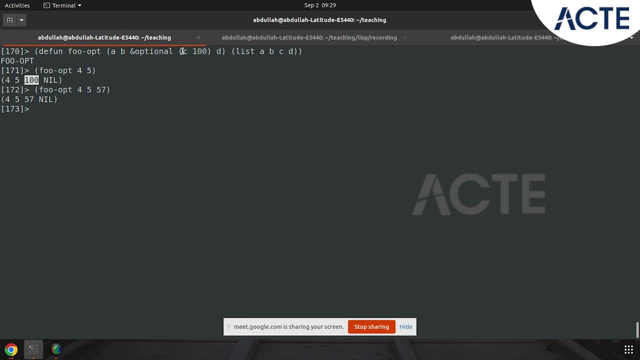 by default, so it appeared as 100. if you do. if you had not put the c, it would have been nil. okay, but since you put c as 100, it has taken 100 and put in here. but if you want, you can put 57, you can. 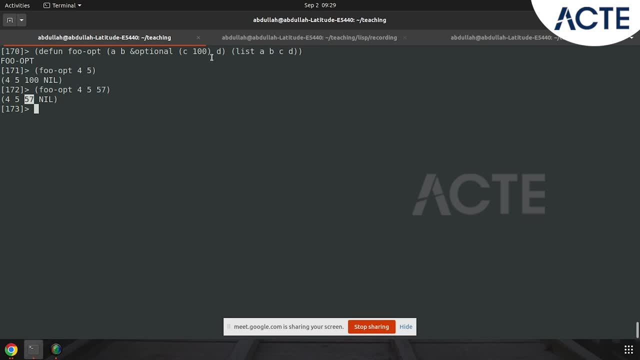 override that uh default value and becomes 57 and d is actually nil and you can also specify a value for d. but the limitation of this guy is you can only specify between two to four parameters. okay, this will not allow you to do it. so if you want arbitrary number of parameters, we have. 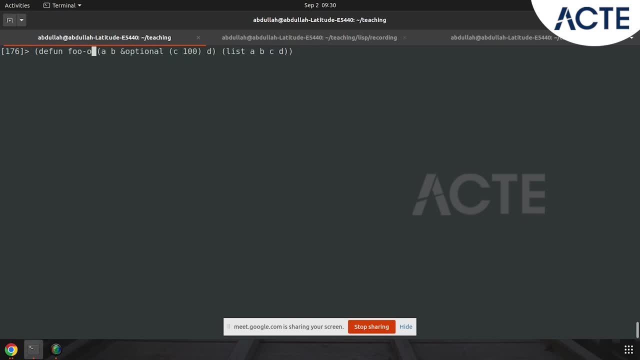 something called rest, right, so something similar to plus or, uh, plus or star. i can say rest, and this will catch all the values. okay, so what this thing does is it requires at least two, okay, and the two values are the same. if it is not two, it will not work as as before, because required arguments are those that are just